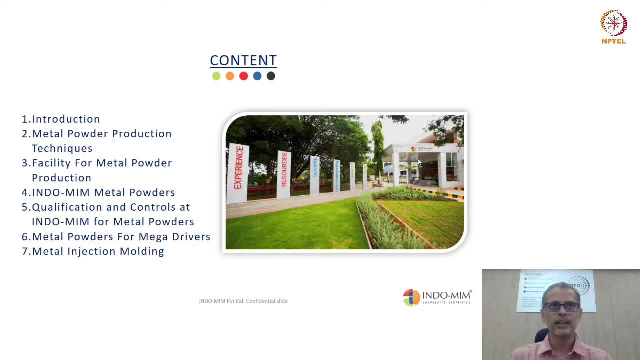 the one which is at Endomim. We are one of the only company having this kind of unique powder production facility. We also talk about Endomim metal powders. that is, what kind of metal powders are being used at Endomim. So we talk about that. We talk about qualification and 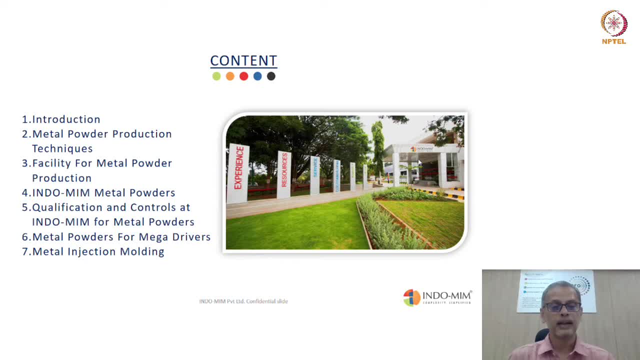 controls at Endomim for metal powders, And we talk about metal powders for mega drivers. So what are the main areas where these metal powders for additive manufacturing have been really catching up? What is the scenario in the industrial market look like? 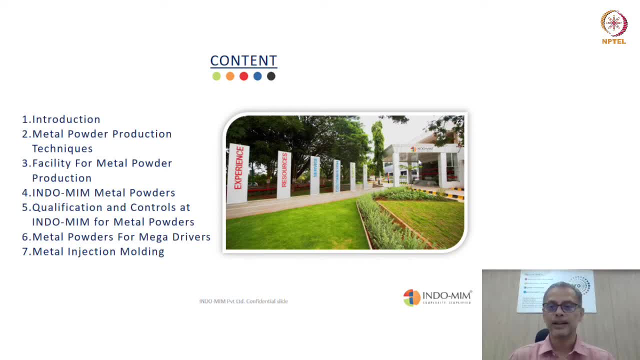 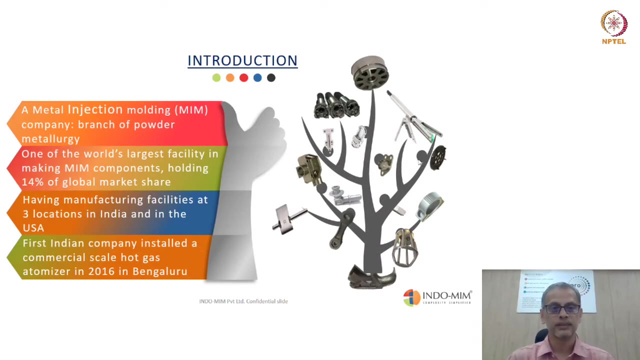 And, of course, we talk about our core technology- metal injection molding- before we close for today. So I hope this kind of content is aligned to your expectations. So let me commence the introduction. So Endomim is a metal injection molding company And metal injection molding 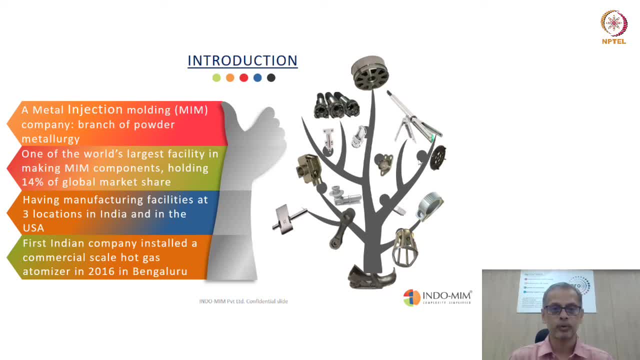 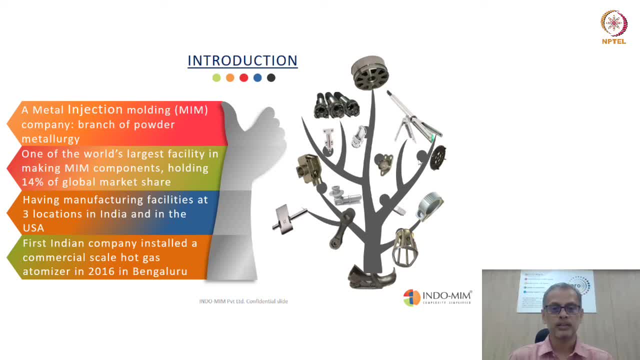 of the branches of powered metallurgy. as few of you might know, We have one of the largest facility in the world to make compared components And we have market share, global market share roughly about 14%. Actually, this entire market of metal injection molding is very, very scattered, you know, So it has a very, very long tail. 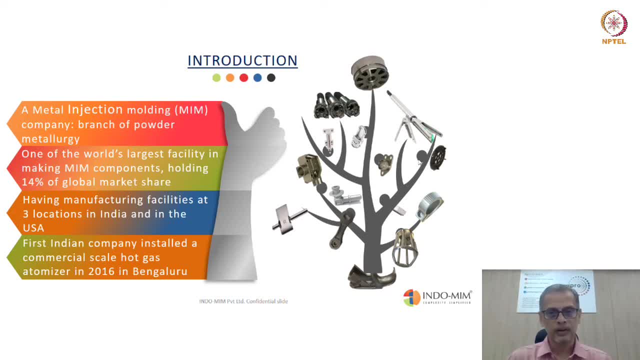 if I may say so, And the lead goes elsewhere And the tread has a machete. the Quick performance tool has the less ground And totally this兄al is the front of Endomimi. There is no, And we are of course the world number one, and world number two is roughly about one. 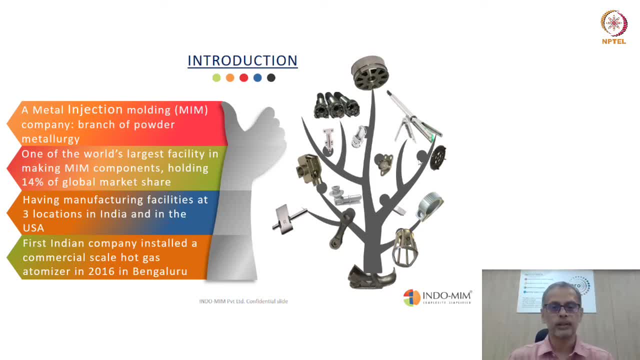 third of our size. And then of course, you have a lot of other companies. there are roughly about hundred companies in China, there are about 50 odd companies in Japan, similar number in Europe, and so on. Indomim has three manufacturing locations in India, two for metal injection molding. 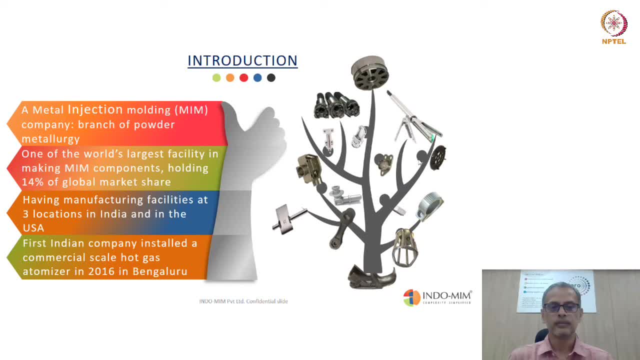 and one for investment casting And we started about three years back also a greenfield metal injection molding plant in USA. We, as I mentioned earlier, are the first Indian company to install a commercial scale hot gas atomizer. This was done about four years back in 2006 in Bangalore at our Dodd-Bellapur facility. 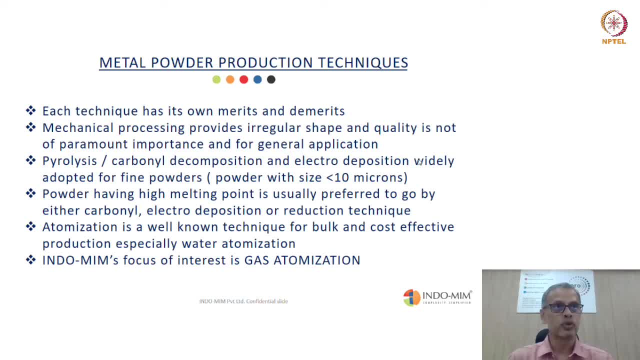 Let us focus some time on metal powder production techniques, because I am sure all of you might be curious as to what kind of metal powder production techniques are used. what are their merits? what are their day merits? why are there multiple metal powder production techniques? 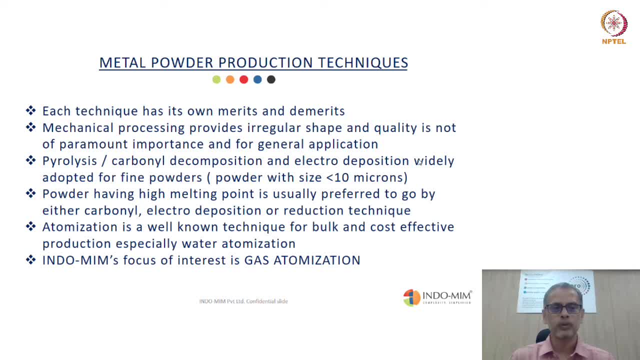 So I mean one thing which all of you probably might be able to visualize or imagine is a mechanical processing, or you also call it milling or grinding of powders. Now, mechanical processing provides irregular shape, and this is something which is used where quality is not of primary. 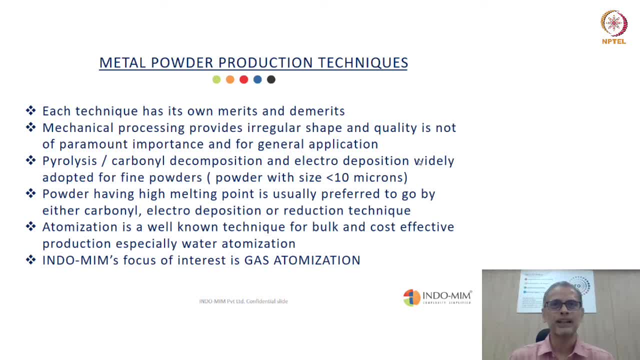 So we have to be careful about that. So we have to be careful about that. So we have to be careful about that. It is not of prime importance. Simple examples that I could cite would be gas cutting or welding application. 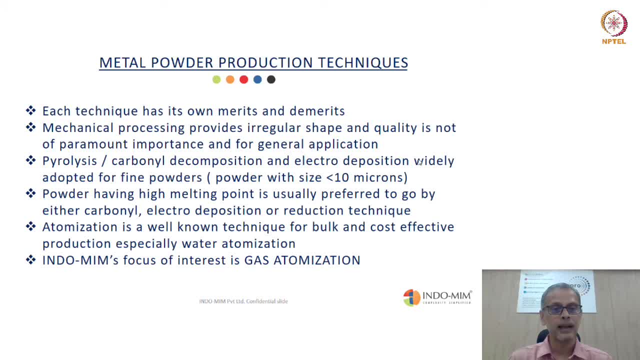 So this is something which is used for mechanical application, and aluminum powder, which is subjected to mechanical milling, is also used in cracking application, So that is another application for that. So predominantly mechanical processing is something which is used where quality is not of paramount importance. 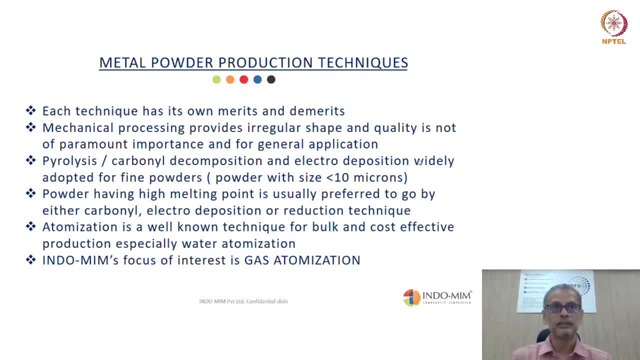 paramount importance and where scale is of importance. So mainly, I would say it is mainly for general applications. The second technique which is pretty popular is called pyrolysis, or I would say carbonyl decomposition and electro deposition. This is used mainly for powder size less than 10 microns. 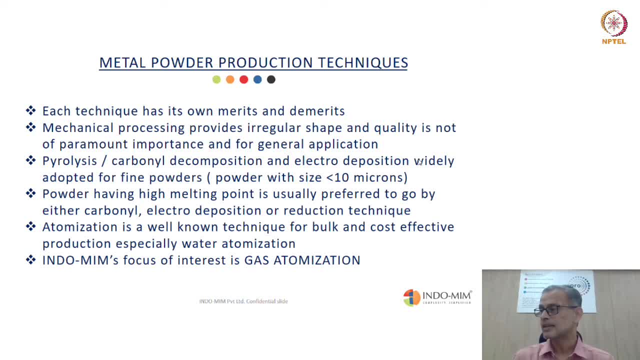 So food industries, iron vitamins, industrial applications- these are some of the applications. and then you have basically molybdenum, which has a melting point of about 2700 degree centigrade. So that is some powder where high melting point is one of the prerequisite for getting 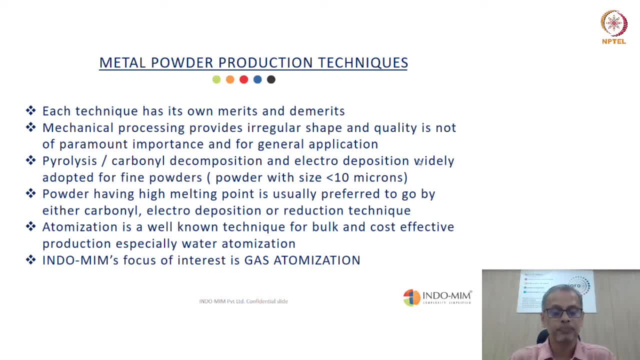 into carbonyl or electro deposition or reduction technique- Tungsten might be another example Which- Which also has a high melting point- and then the carbonyl root is something which is used for production of such powders. And then the other thing that you do in atomization and the other technique that you do, very popular. 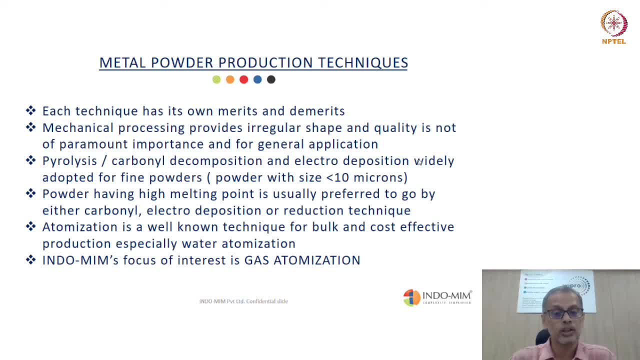 is called atomization, which is mainly for bulk or cost-effective production, And within atomization, there are two types: One is water atomization and another one is gas atomization. So water atomization is something which is pretty popular And again, a simple example could be iron powder. iron powder, which is usually made by water, 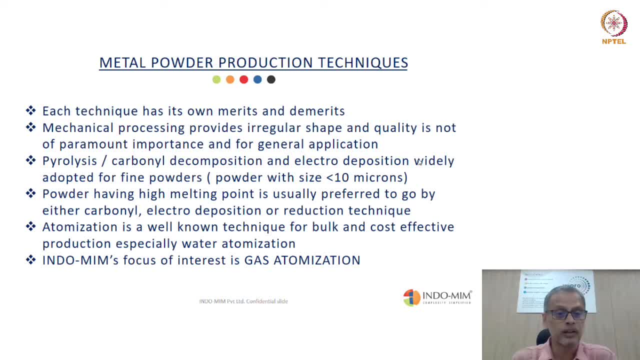 atomization, where of course you get irregular shape. in water atomization You get. basically you have to do additional operations like de-watering, like drying, which of course consumes some time, But ultimately you end up spending a lot less amount of expenditure as compared to gas atomization. 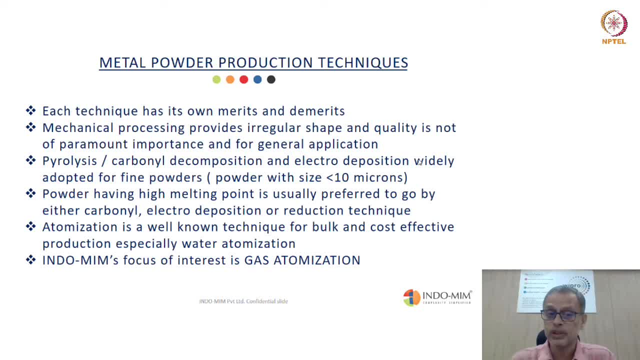 Right? So water atomization is a technique that produces a bit of irregular shape, and it again can be used for areas where oxygen content or nitrogen content is not very, very important, Right? So what is happening here is that there is a pick up of oxygen and nitrogen content from 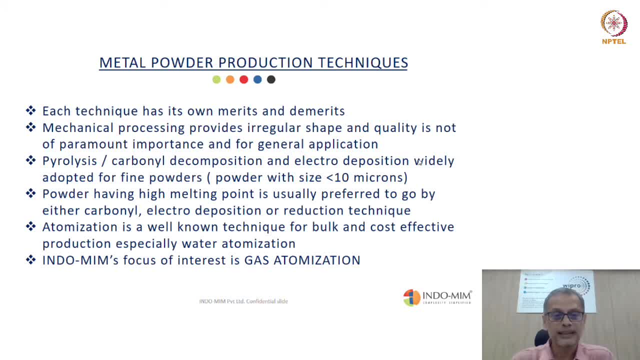 water or even hydrogen content from water, and that is something which remains in the powder when you use a water atomization technique. Right, So these basically I can call these as impurities. presence of oxygen and nitrogen and the applications of water atomization, typically iron, are areas where you may not want these impurities. 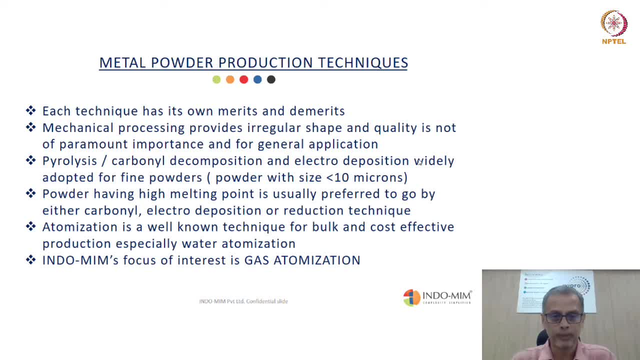 to be below a threshold level of a few ppm, Right. So the technique which Indomim has been focusing on is called gas atomization, and gas atomization is predominantly a technique where you would have these ppm of all hydrogen, oxygen, nitrogen, to be below something like 100 ppm. 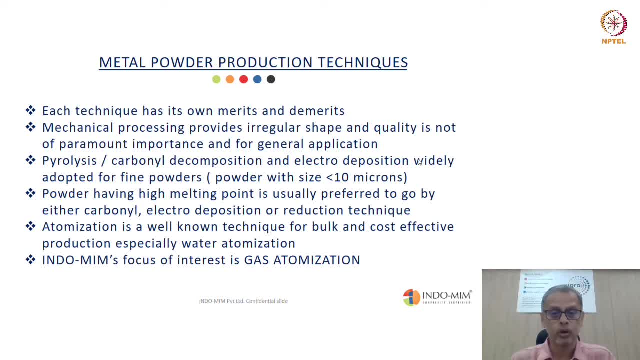 I mean there are techniques available where you can even control them below 100 ppm, and there are various applications, starting from aerospace or starting from medical devices or even oil and gas. There are various sectors where these kind of gas atomization techniques or production methodology is used, because you have a very, very clear focus on controlling the ppm levels. 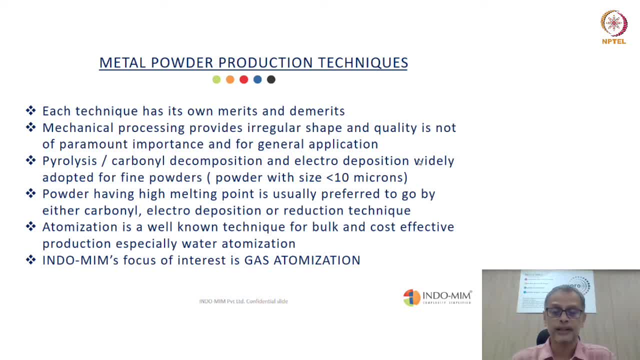 of these impurities because these are going to affect the end product quality in a direct way. So at Indomim we have been focusing on utilizing this gas atomization process As well as further perfecting it, such that we are able to give the product of quality. 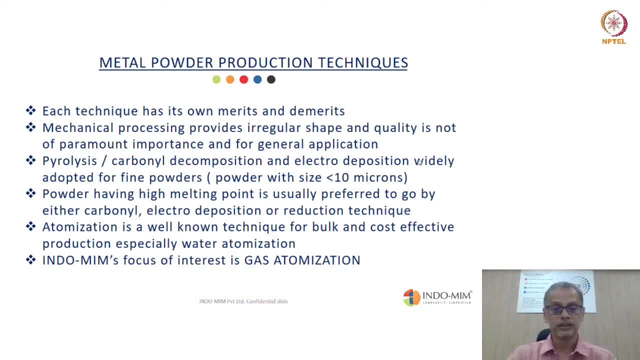 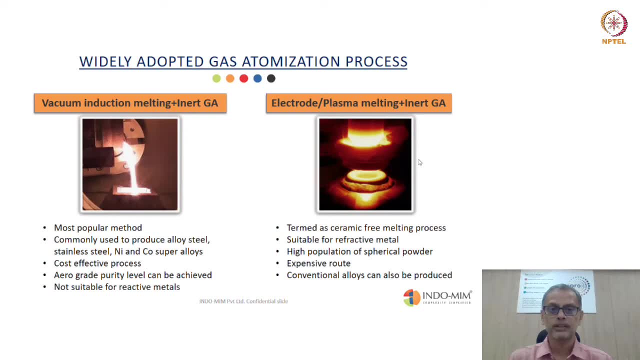 as required by these demanding industries. So delving little bit further in gas atomization process, which is widely adopted, it can be the gas atomization process can be implemented or the production can be done using two specific methods. One is vacuum induction melting plus inert gas, of course, and electrode or plasma melting. 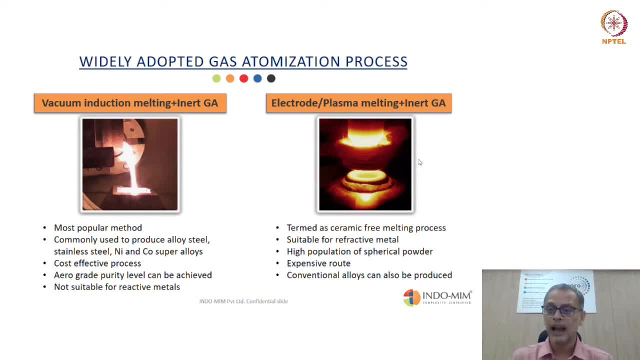 as it is also called, plus inert gas atmosphere. So basically, we have inert gas as an important element in both these processes, But the specific discrimination- as you can see on this slide- between these two processes is that one is using a crucible, whereas second is not using crucible. 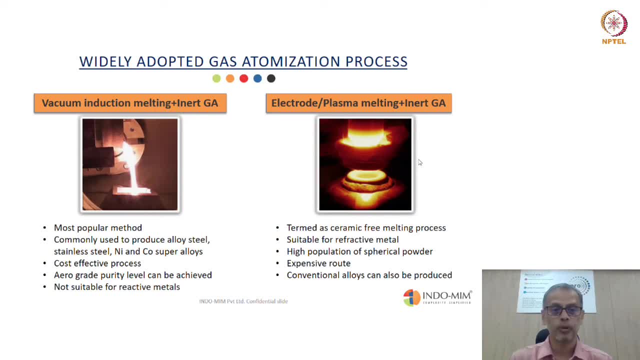 So vacuum induction melting is something Which is one of the most popular method that is used for producing most of the alloy steels, stainless steels, nickel and cobalt super alloys. It is basically a process whereby you have a crucible into which this particular molten. 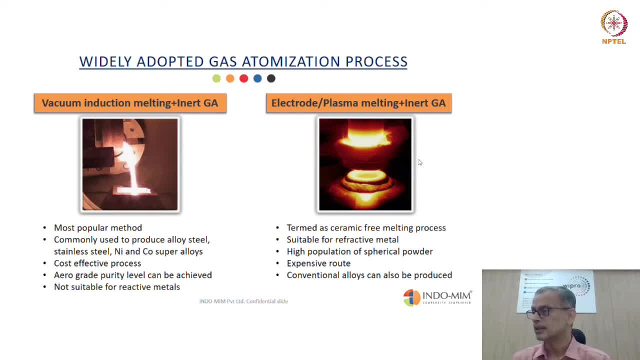 metal is poured And the crucible is mainly having some amount of silica or aluminum oxide which probably would get mixed up with the molten metal There by, Because there is some gas which gets eroded and mixed. and these are some of the inclusions. 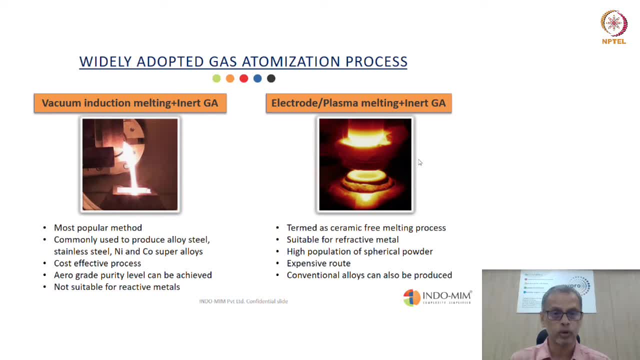 which may be present inside the molten metal while it is getting atomized And it can certainly achieve a aero grade purity level, but not to the. I mean I would say about 70 percent of the applications of aerospace would be utilizing this kind of. 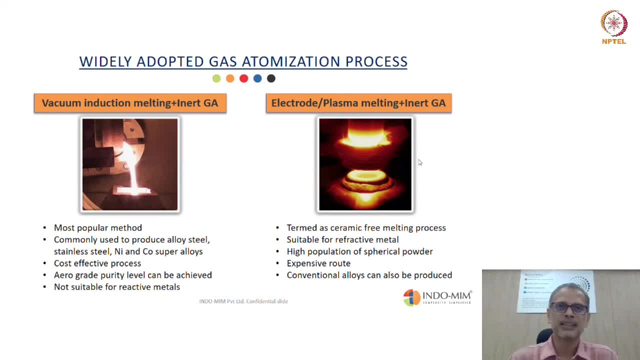 vacuum induction melted gas atomization process, whereas some of the demanding applications, probably 25 to 30 percent, would be using this kind of vacuum induction melted gas atomization process. So the crucible might not be able to use the product out of vacuum induction melting. 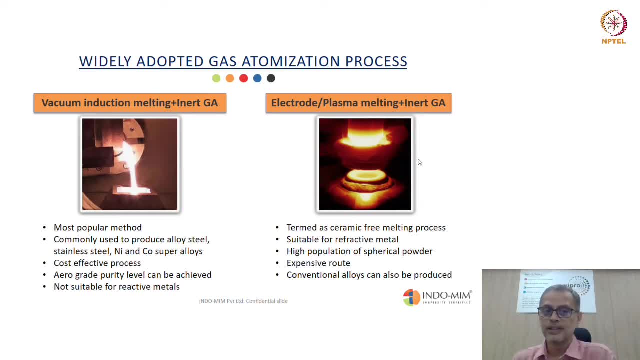 and also it is not suitable for reactive metals. So, in summary, vacuum induction melting has a crucible. it enables some of the impurities or the parent material of crucible to be mixed along with molten metals. while it is being, the molten metal is being poured and it is used for about 70 percent of the aerospace. 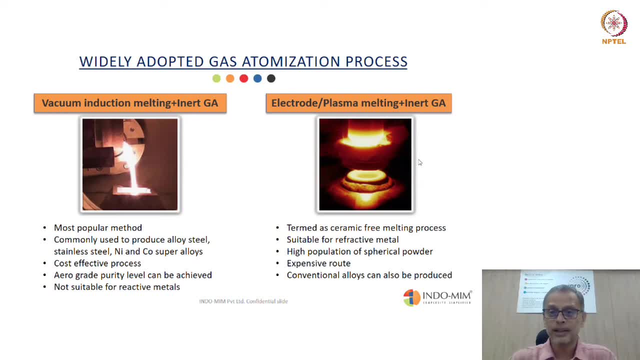 applications. Coming to electrode or plasma melting again here, as I said, it has inert gas and it is termed as a ceramic free melting process. it is used mainly for refractive metals. The simplest thing here is that the inclusions which normally come because of the presence 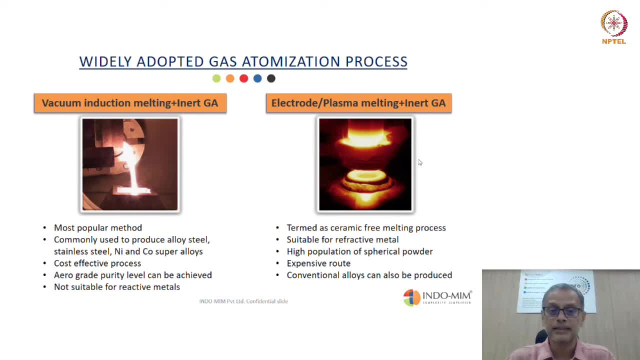 of crucible are going to be absent here and that clearly indicate that you would not have impurities, And hence the population of squalene. So this is the crucible, So this is the crucible, So the population of spherical powder is going to be more. 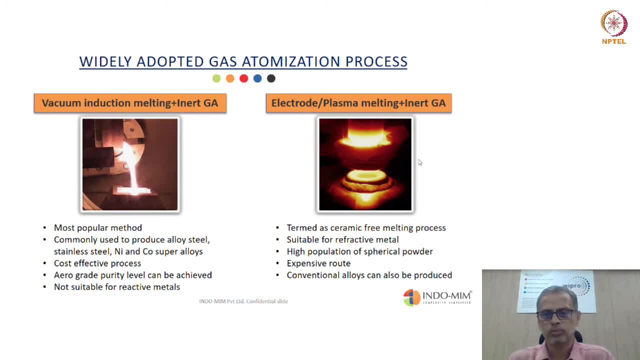 Certainly this is an expensive route, but then if you have any conventional alloys also to be produced here because of this purity content or because of this higher population of spherical powders, it is definitely preferred. The highlight here is that the electrode that itself acts as a crucible here. 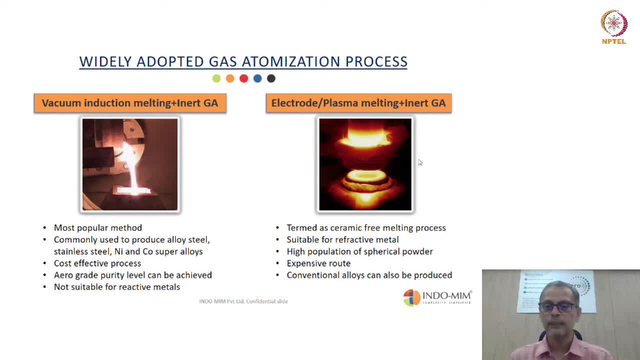 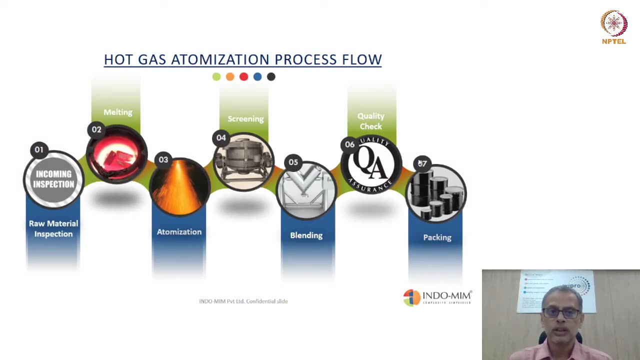 So this is the crucible- no formal ceramic crucible that is used here, since it is a ceramic free melting process, but the electrode itself acts as a crucible and the melting process takes place using this plasma. So let us come to the hot gas atomization process flow. So this slide briefly explains you the 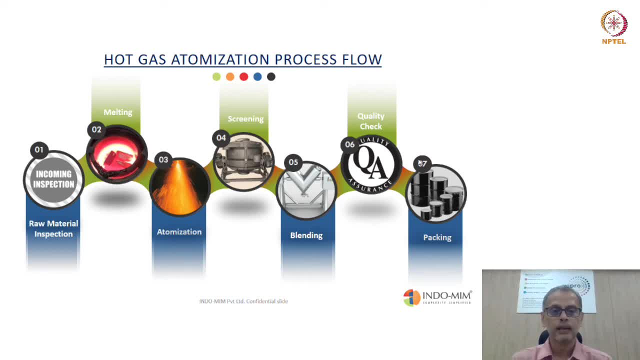 process flow that is being implemented at Indomim. So we have basically the seven-step process which is given in this flow chart. The first, as you would obviously understand or appreciate, is incoming inspection. So the raw material is coming into the plant. there is a formal way of. 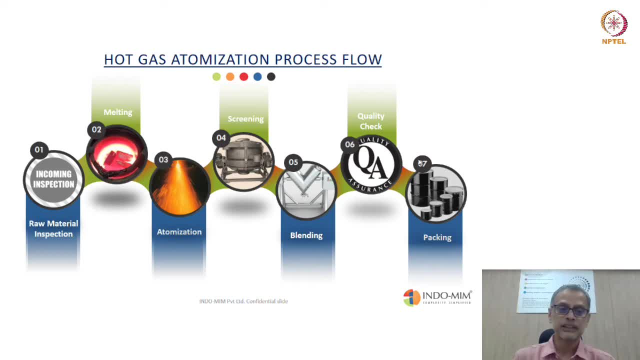 incoming inspection, which is done. The second process is melting, right. So melting is where the molten metal is poured, and this we have something called a Tundish process, whereby there is a large vessel in which there is a small orifice at the end. So it will be poured from the crucible into this tundish and 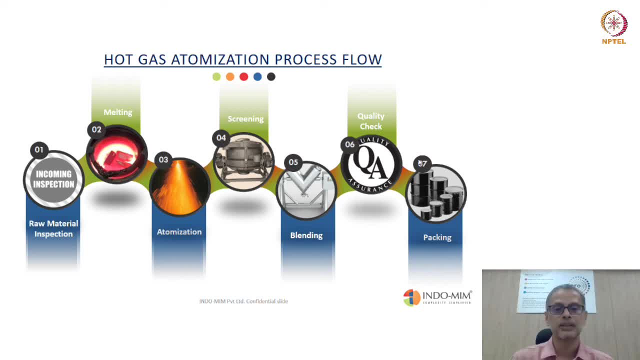 this allows the flowability of the molten metal through this small orifice about 6 mm or so, before it goes for the atomization process. Now, friends, what happens in atomization process is that there is a gas which flows at a velocity of something like 1 or 1.5 Mach. 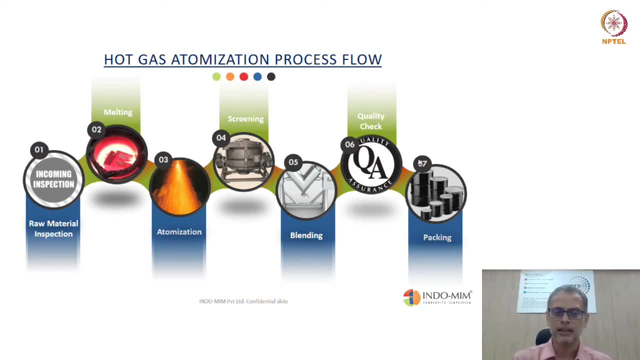 right 300 meters per second or something, and under that high pressure, when this 6 mm orifice is leading some hot molten metal into the large vessel, that is where this atomization takes place. So the facilitation of atomization is taken place through the high velocity of the inert gas. 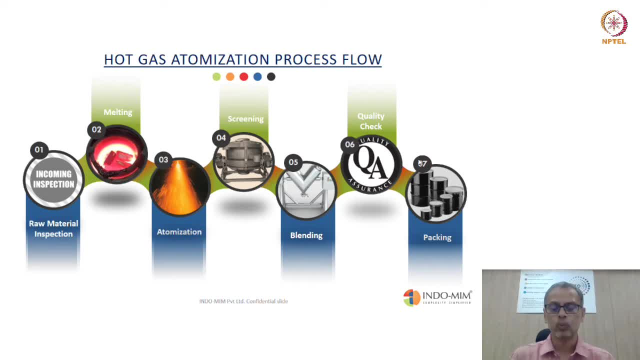 right and once the atomization is done, what you have as a result of it is probably particles less than 5 microns, going up to about 150-200 microns. So it is a very-very wide array of particles that would come as a result of atomization. So, necessarily, what we need to do is 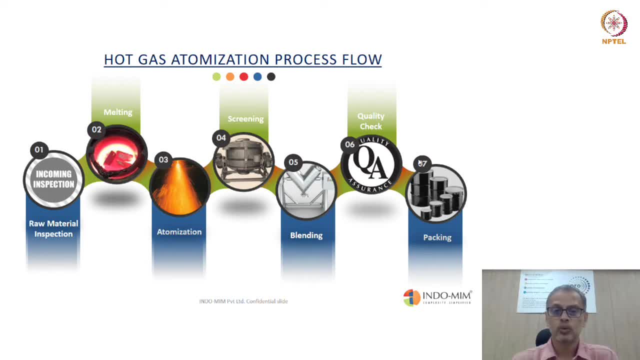 we need to screen them. The next process is screening. So what do you mean by screening? Screening is basically classification of these powders into different size levels. So we have, for instance, less than 20 microns, which is used for metal injection molding. 20 to 50 microns is 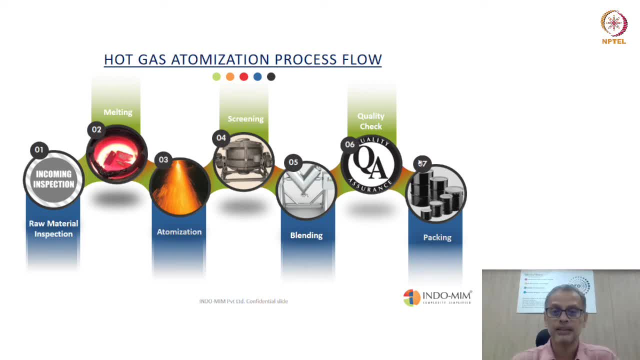 used for some of these additive manufacturing processes. The most popular band for additive manufacturing is 50 to 150 microns and, of course, beyond 150 microns is used for other processes. So the major powder that is being used is between this 0 to 150 microns, and that is something which 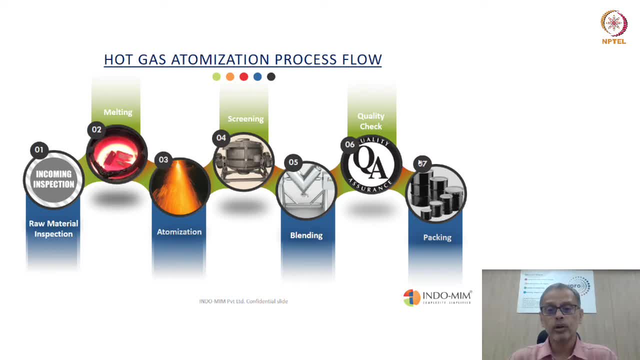 is done through this screening process. Subsequent to that, we have blending process, again where our team has done some wonderful work of establishing fine processes that enables us to have very good blending, which subsequently goes to the quality check. So quality assurance is the area where we do this quality check. So we have various in-process. 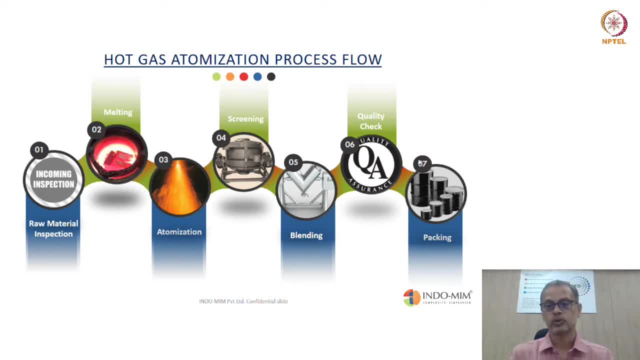 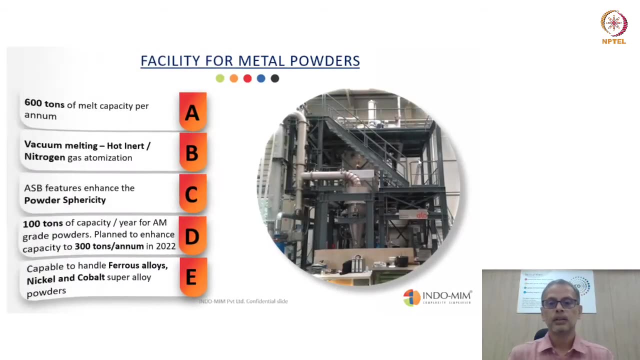 inspection stages while we go through these processes. but, of course, quality check at the end of the completion of blending is something which is done before we pack these products Into predetermined boxes or predetermined packaging sizes. So here is an image of the large scale hot gas atomizer that is available at Indomim. 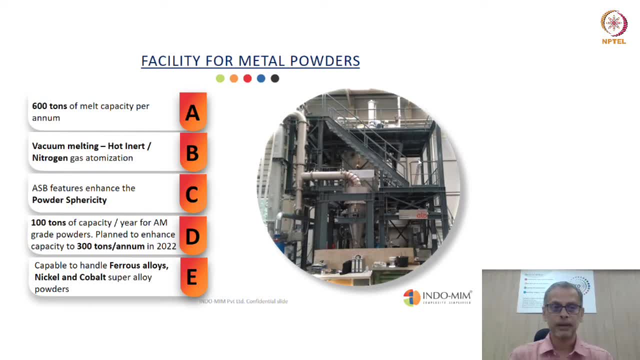 We have a melt capacity of about 600 tons per annum, and this is, of course, vacuum melting or hot inert nitrogen gas atomization process. I will talk about ASB features- anti-satellite features- that our team has wonderfully worked along with the supplier to have this kind of. 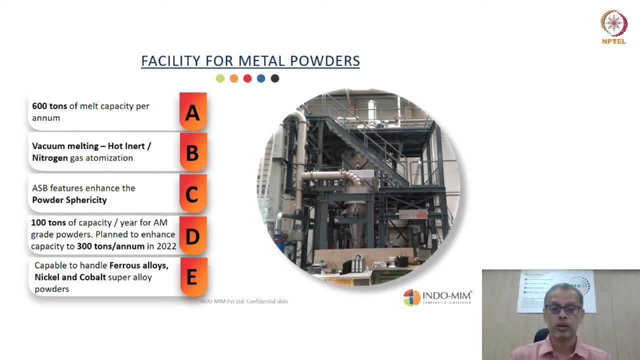 feature that is mainly helping us to have very good powder sphericity. and on additive manufacturing we are focusing a lot. Currently we have about 100 tons of capacity dedicated for additive manufacturing out of the 600 tons that we have and we are planning to enhance. 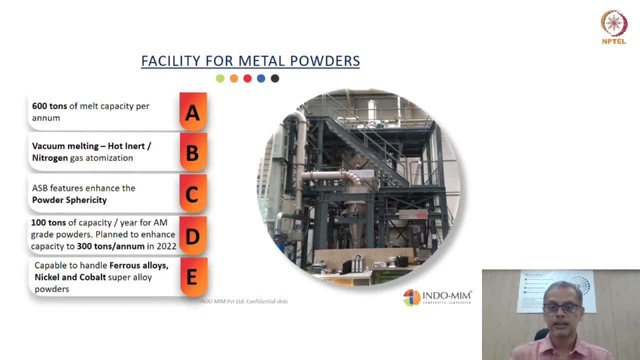 this capacity to roughly about 300 tons per annum by the year 2022.. Currently we are able to handle ferrous alloys, nickel and cobalt super alloy powders and we certainly plan to get into new and new varieties of powders based on the demands from our additive manufacturing. folks across. 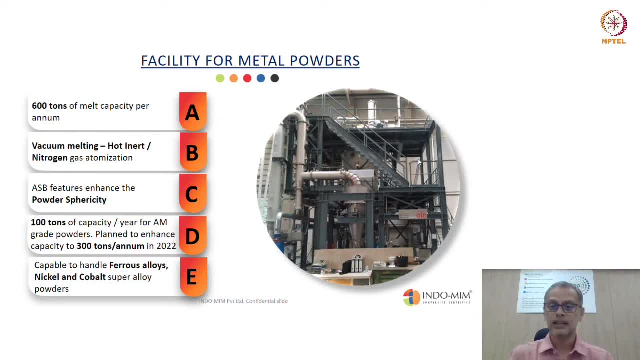 the country as well as internationally. I am very pleased to say at this stage that majority of additive manufacturing shops in the country today have switched over to Indomim powders and they are pretty happy and pleased with the performance of our team, both the technical as well as the commercial team. I mean just to say that the pricing wise. 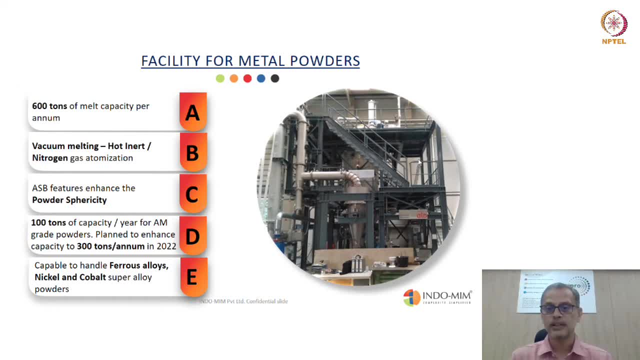 we are competitive and we are also able to support most of these additive manufacturing shops with respect to specific powders that they need, with respect to R&D efforts that they need. Many times they need specific controls on flow rate at their end. So to enhance the print. 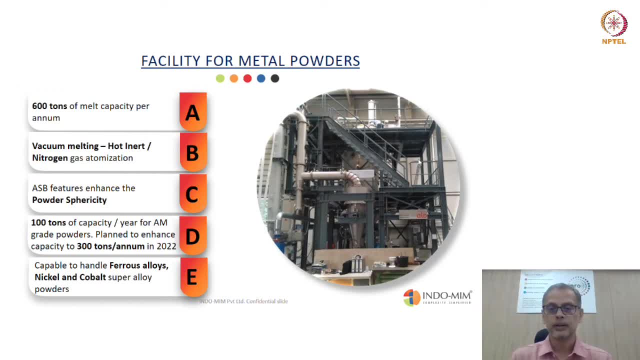 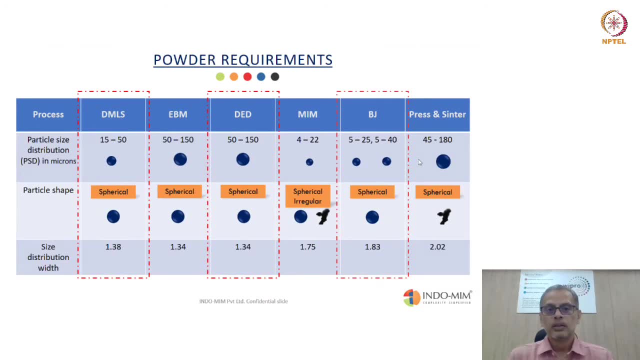 quality. we have been able to do a good work with respect to providing them the right technical support in terms of a powder manufacturer. So, expanding further when we talk about the powder requirements, as you all know, there are multiple additive manufacturing processes. 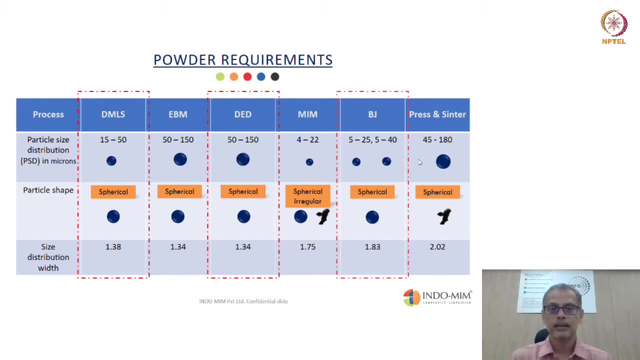 starting from DMLS, EBM, DED- majority of them- and then, of course, we make powders for metal injection, molding, as well as binder jetting and press and sinter. Press and sinter is the routine powder metallurgy, age-old process. So in the second row, friends. 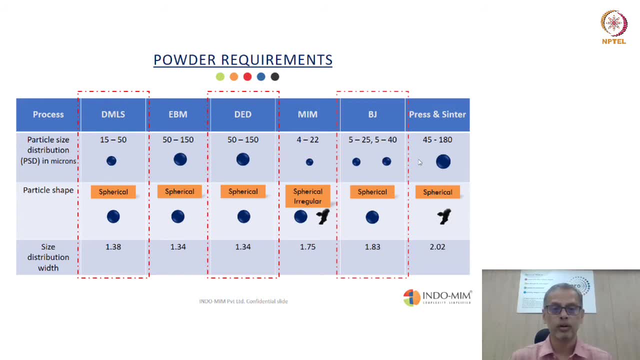 you can see the particle size distribution in microns that is given for all these different kinds of processes. For instance, DMLS- direct metal laser sintering uses 15 to 50 microns. EBM- electron beam uses 50 to 150 microns. Same is the range of particle size distribution used. 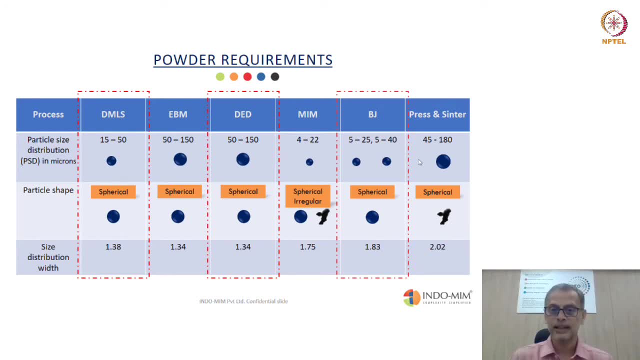 for DED Metal injection. molding, as I said earlier, uses less than 20 microns, so roughly about 4 to 22 microns. So we have a total of about 4 to 22 microns. And binder jetting is another very interesting process that INDO-MIM has got into in the 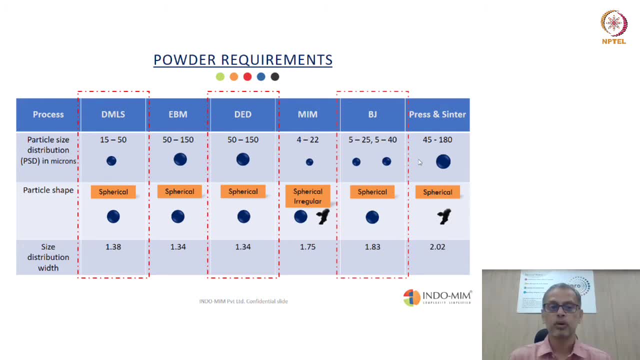 last 18 months or so, where again, the powder size that is used is about 5 to 25 microns, or going up to 40 microns in critical cases. Beyond 40 microns, that is, from 45 to 180 microns, is something which is used for press. 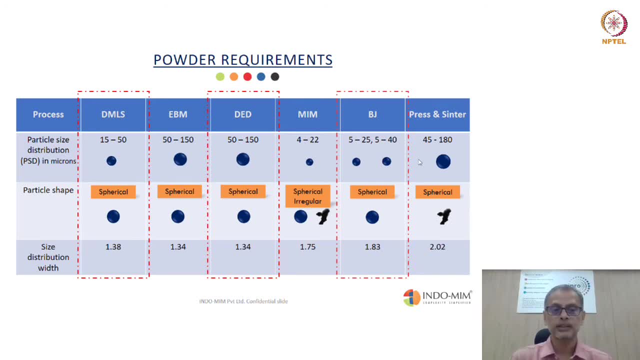 and sinter. So the third row, as you can see, is about the particle shape. So majority of additive manufacturing requires a spherical shape. That is one of the important requirements for having a better printing quality, whereas metal injection molding uses spherical or irregular shape. 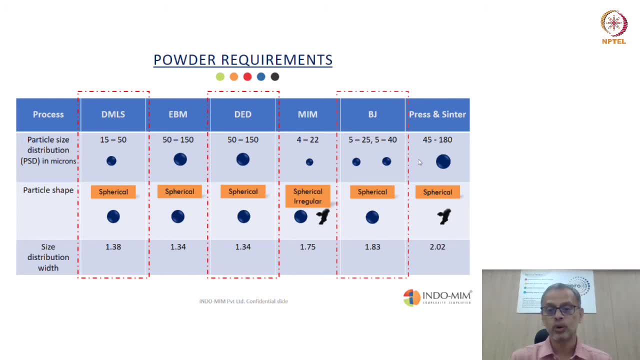 You need to have a combination of these shapes. That is something which enables you to have a better packing in metal injection. molding, Binder jetting also requires spherical shape and, of course, in coming to press and sinter, you have combination of spherical And irregular shapes. 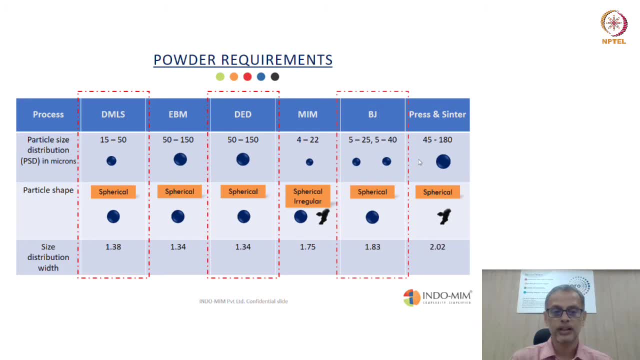 Size distribution width is something which I would like to draw attention from all of you. That is the fourth row, which clearly highlights what kind of size distribution width is something which is used for various additive manufacturing processes, as well as metal injection, molding, binder jetting and press and sinter process. 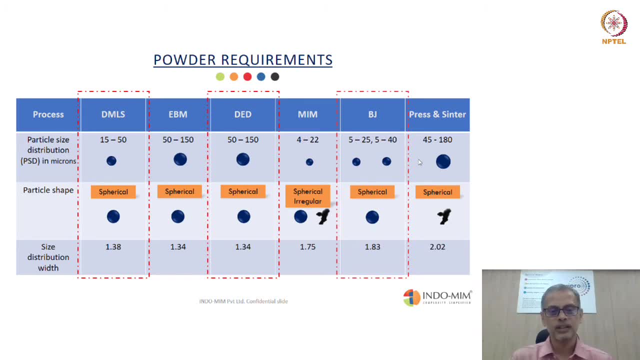 So you would see that typically additive manufacturing oscillates. So you would see that typically additive manufacturing oscillates. It oscillates between about 1.34 to 1.38 as far as the size distribution width is concerned, Whereas when we go to metal injection molding it is reasonably higher: 1.75, binder jetting. 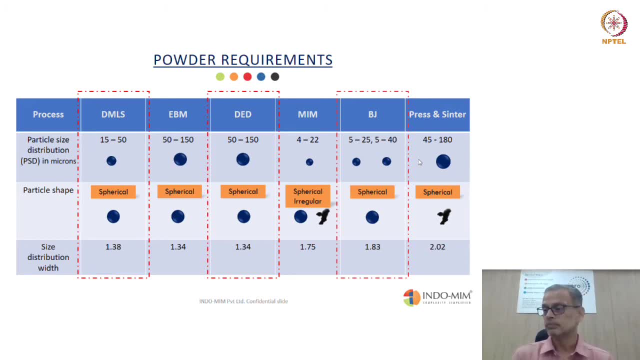 again going higher to 1.83, and of course, the press and sinter uses about 2.02 as the process or the size of distribution width, That is 2.02.. So this is the first row. So I would draw your attention to this size, distribution width, because this is something. 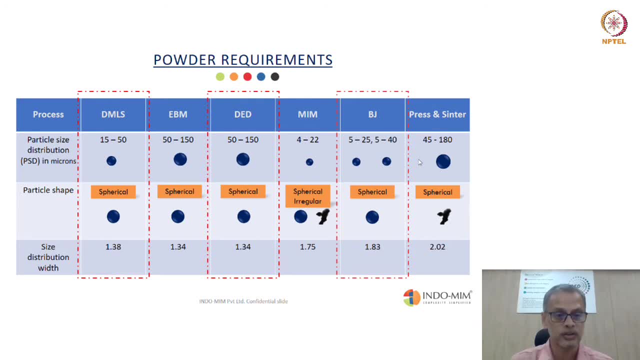 which additive manufacturing focuses on. So typically for additive manufacturing we need little- I would say narrow distribution that directly affects the print quality. So you can see in this chart that 1.34 to 1.38 is the size, distribution width that has. 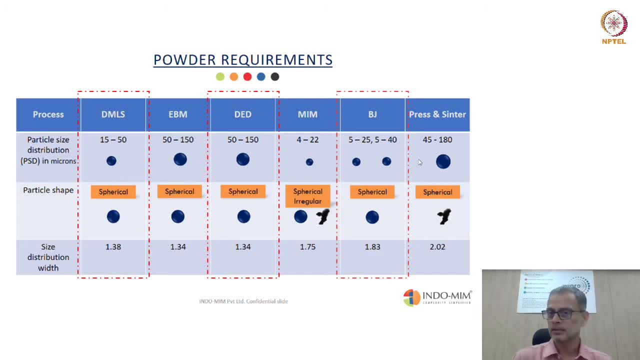 been used. So this is the size distribution width for additive manufacturing. Again, to highlight little further, in case of metal injection molding you have a higher size distribution width. Again, there is a reason for it, because by having this you are able to have a better 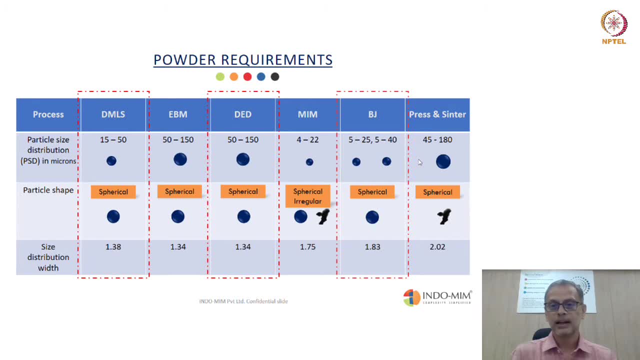 I would say packing, in terms of molding process and other things. And binder jetting, if you would know, is also very similar to metal injection molding, just that the molding element of metal injection molding gets replaced with printing in case of binder jetting. 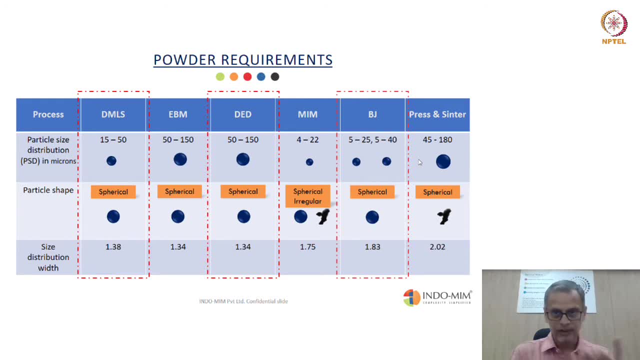 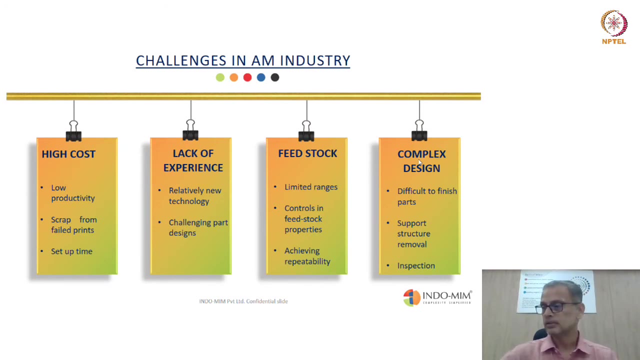 Whereas the debinding and sintering processes that I will explain little further when I go to metal injection molding is also present in binder jetting Challenges in the AM industry. I think all of you probably are aware that additive manufacturing is certainly going through a lot of difficult times. 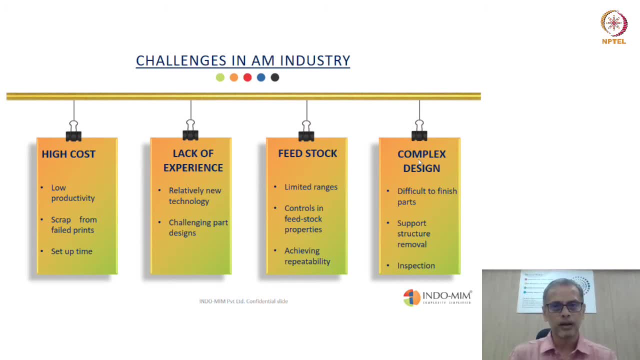 I mean it was definite. there was definitely a hype about additive manufacturing catching up very quick. but then there are mainly these four challenges which are mainly affecting most of the job shops or 3D printing shops: high cost, lack of experience, feedstock. 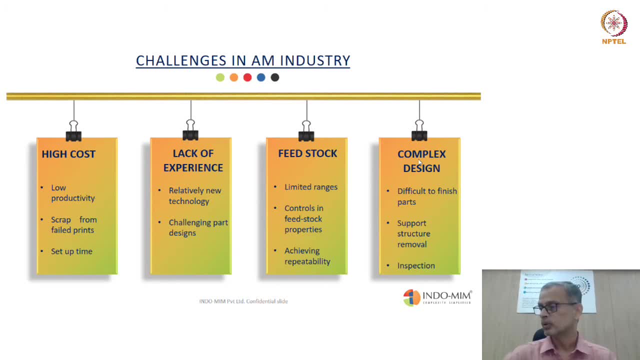 complex design. So these are the main four things which are going to be affecting the growth of additive manufacturing industry. When we say high cost, it is basically the manufacturing industry. It is the manufacturing industry. It is basically because of low productivity, as you would all know or probably imagine. 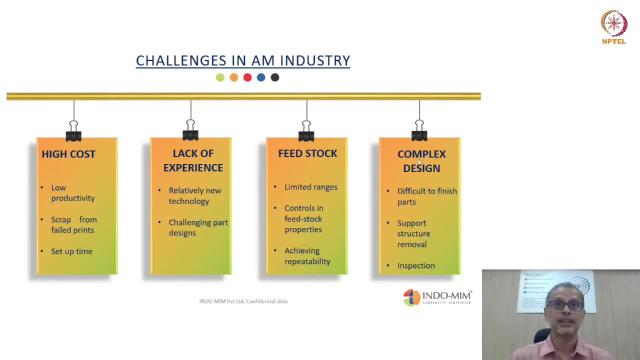 The other reason also for high cost is scrap from failed prints. So basically the yield that is coming out of additive manufacturing process is not very good owing to the failed prints. And the second important thing is the setup time. So these are the three main elements which are contributing to high cost in the additive. 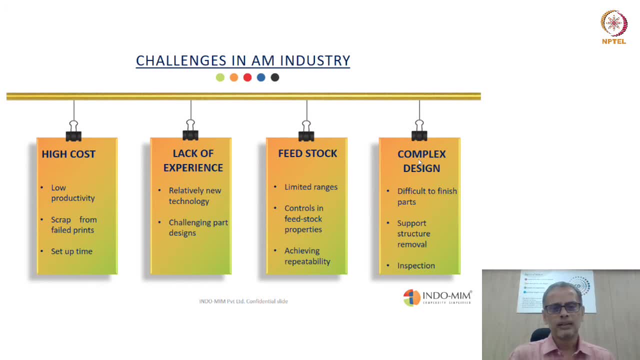 manufacturing process. I mean, it is a relatively new technology. I am sure all of you know that additive manufacturing is a very, very advanced technology. Additive manufacturing is not very old in terms of technology, although there has been a lot of research going on, especially in the West. 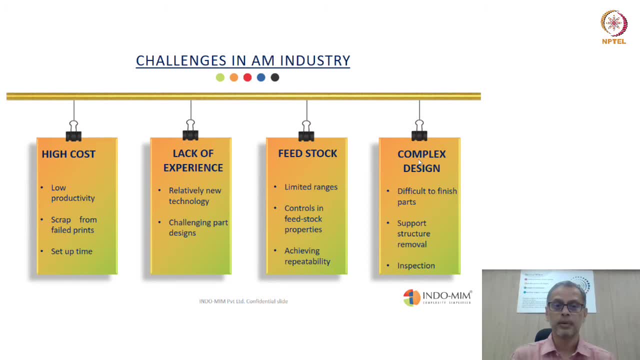 And the second important area, why additive manufacturing is struggling owing to the factor of lack of experience, is the challenging part. I mean, I am sure you know that aerospace is something or oil and gases are two industries which are trying to utilize or I would say, exploit, the additive manufacturing technology. 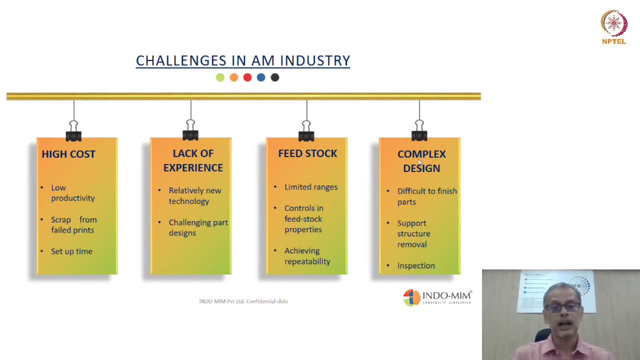 to a very large extent And hence Most of the designers are being allowed to make as much challenging part design as possible, And most of the additive manufacturing shops are having difficulty in producing these part designs. So these challenging part designs are one of the reasons that is causing additive manufacturing. 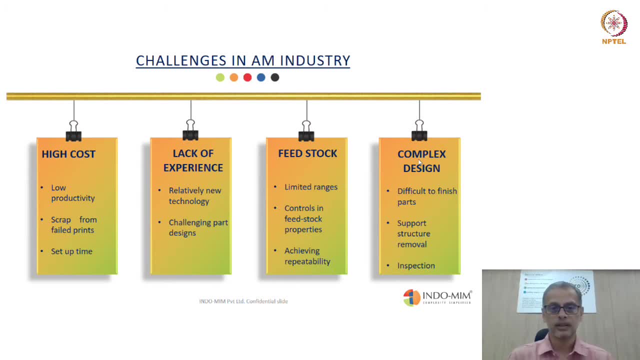 shops not to be quite successful. That is, of course, acting as a challenge. Feedstock: This is another area which is an important challenge. So this is another area which is an important challenge. This is another area which is an important challenge. 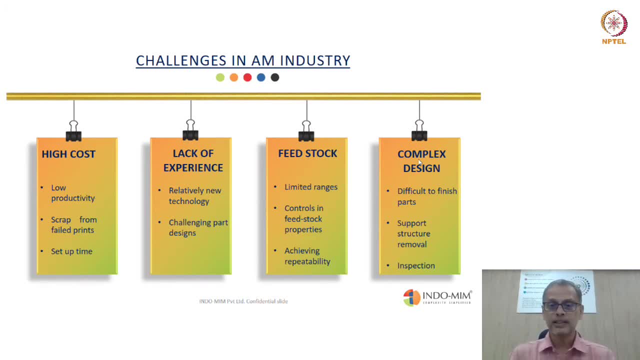 But mainly being focused by Indomim, our company. There are limited ranges, as you would know, in terms of feedstock. The controls in feedstock properties is something which is critical, mainly with respect to achieving repeatability. I would come a little further on talking more about how Indomim has really focused more. 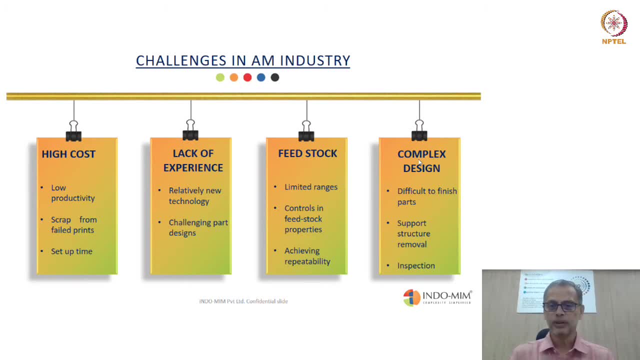 on getting this feedstock thing done And we have been able to support, of course, our own captive requirement as well as most of the customers. The fourth, fourth and final challenge in industries of complex design. So basically, we have difficulty in finishing the parts. Most of you would know that additive manufacturing does not give a very 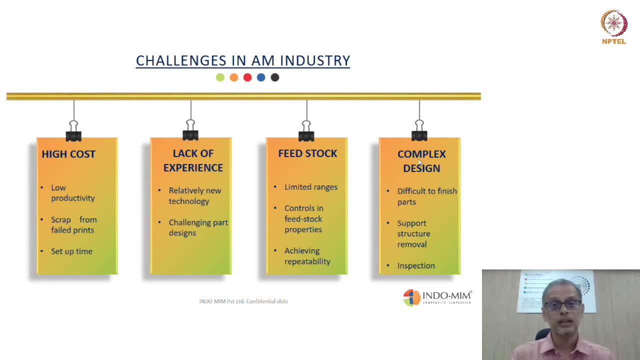 good surface finish, So we need to necessarily have a post additive manufacturing finishing process. The support structure removal is an element which has to be necessarily done, irrespective of what kind of additive manufacturing process we do, and, of course, inspection is an important element that takes up a lot of time. So these are the three parameters. 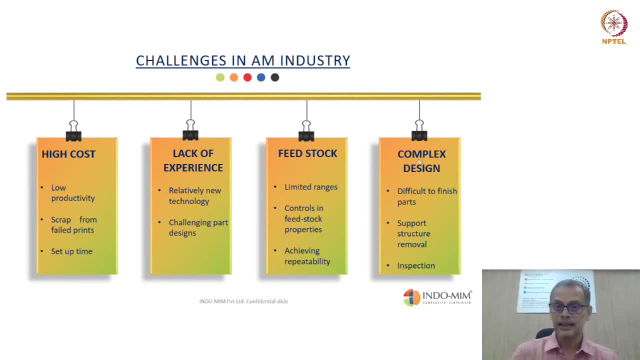 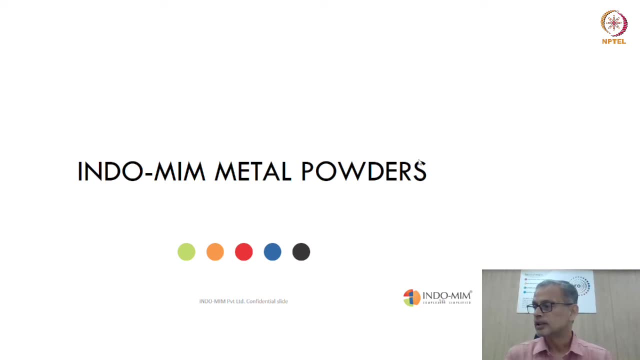 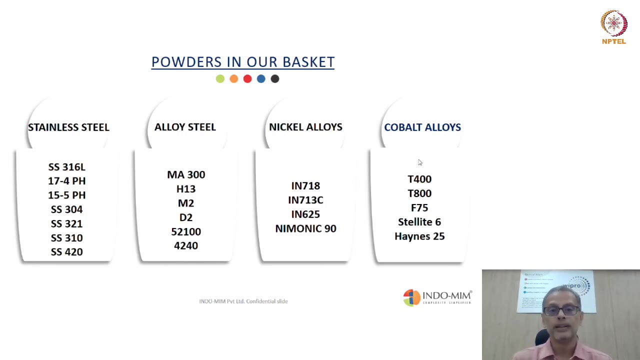 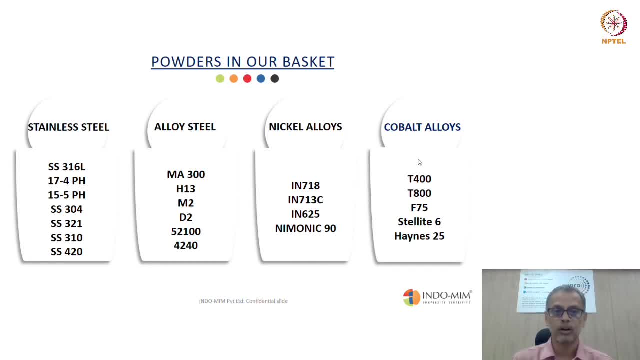 in our industry and what are the parameters that we have included in our industry. So we have basically four categories, or four basic heads, under which we are manufacturing powders and supplying to the additive manufacturing industry. One is stainless steel, where we have almost all. 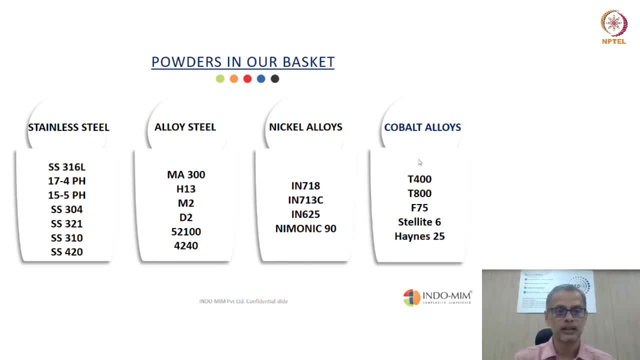 the major fast moving stainless steel items under this particular group: SS316L, 174PH, 155PH, SS304,, SS321, SS310 and martensitic stainless steel- SS420.. So these are the main fast moving stainless steels that we are producing. 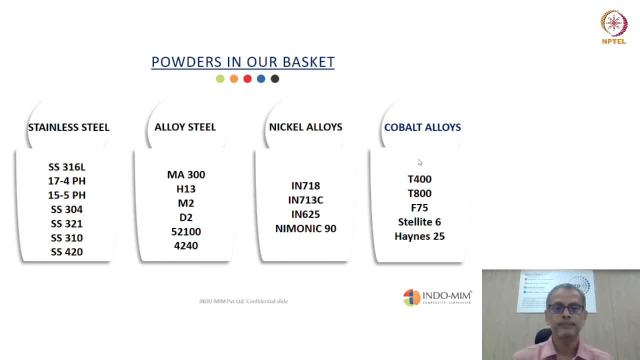 regularly and we have stocks of these powders at all points of time. When we come to alloy steel, we have been making MA300, H13, tool steels like M2 and D2.. We make bearing steel- 52100- and we also make 4240.. So these are the alloy steels, again based on the research that our sales. 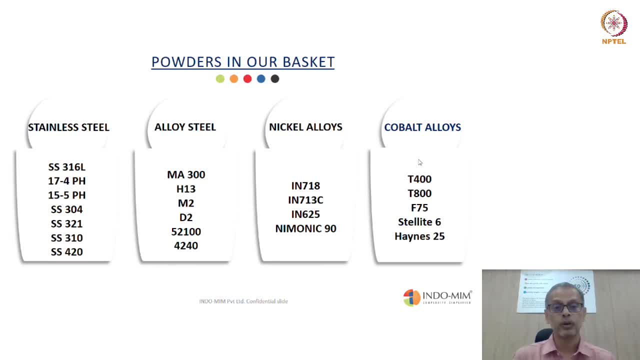 and marketing team has done with respect to what kind of powders are required in the market, These kind of items have been used. Nickel alloys is something which is one of the fast moving product categories at Indomim, mainly used by aerospace applications, as well as some of the 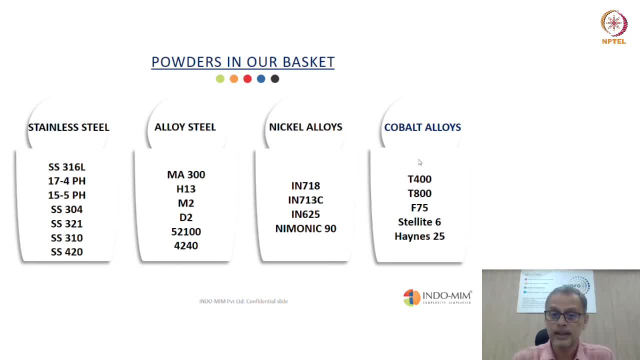 oil and gas applications. So IN Inconel 718, Inconel 713C, Inconel 625 and one of the very popular method or popular powder that we have made is called Naimonic 90. So these are the. 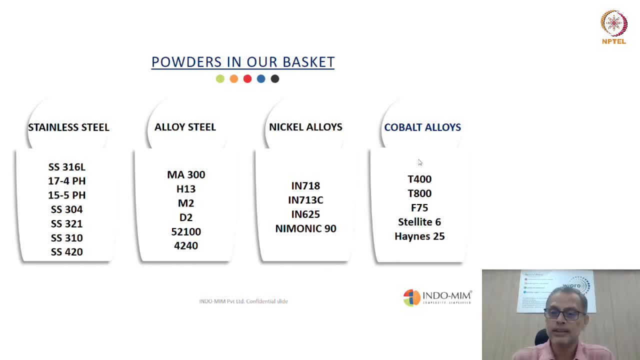 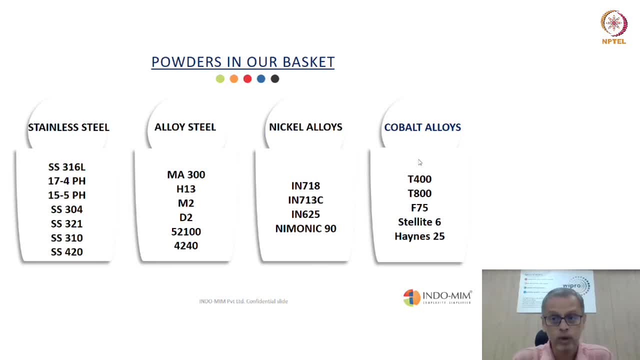 T400, T800, these are the commercial names that we are doing. These are high cobalt powders mainly used for high temperature applications. We are using F75 also as one of the powders- high cobalt, high cobalt chromium, which is used for medical grade. We do produce Stellite 6 and of 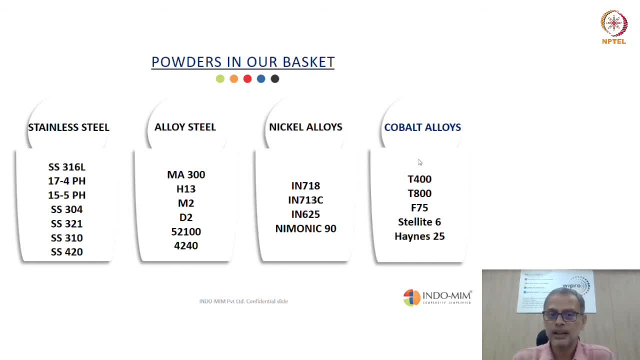 course, we are producing Haines 25 also. So these are the four broad categories of powders that we are making, and I have also made a few of them. So these are the four broad categories of powders. I have also narrated all the specific names of the powders, So this is something which will help. 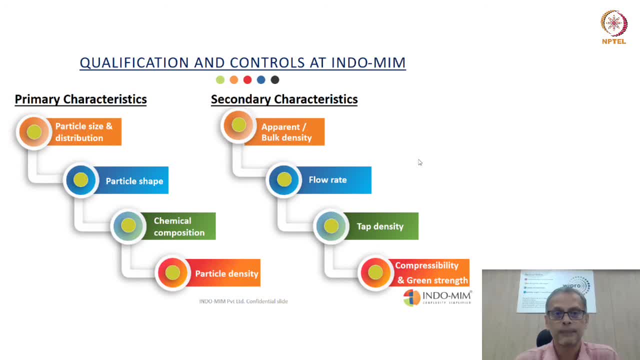 you to remember the variety of these powders. But, of course, producing powders is just not enough. What is important is qualification and controls. So let me take some time and explain to you what kind of qualifications and controls are available at Indomim. So, in brief, these are the four. 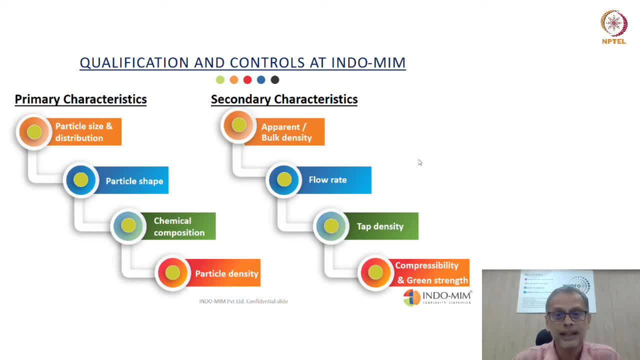 primary characteristics as well as the four secondary characteristics that are being controlled at Indomim. So, in brief, these are the four primary characteristics as well as the four secondary characteristics that are being controlled at Indomim. So what you would see is that 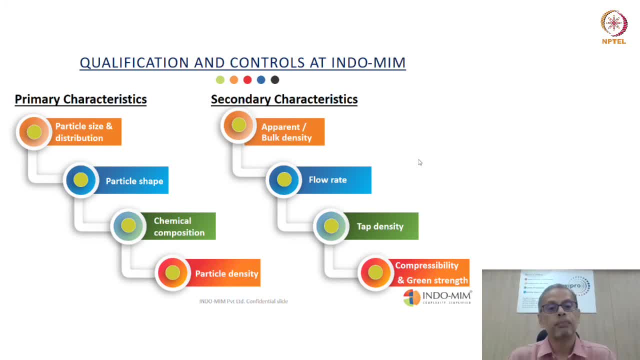 the primary characteristics are particle sizes and distribution, particle shape, chemical composition and particle density. So these are the four primary characteristics that Indomim focuses on, which, in turn, helps us to control the apparent or bulk density, flow rate, tap density, as well as compressibility. 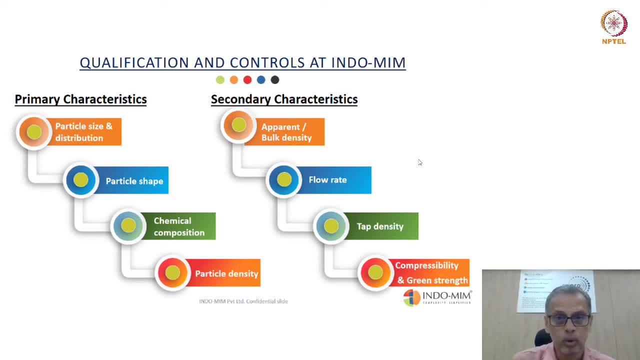 Green strength. So, as you would appreciate that the quality control is something which is important for us to get the powder to the additive manufacturing folks, whereby they are able to utilize them in a better way, and the properties which are listed down here. these are something 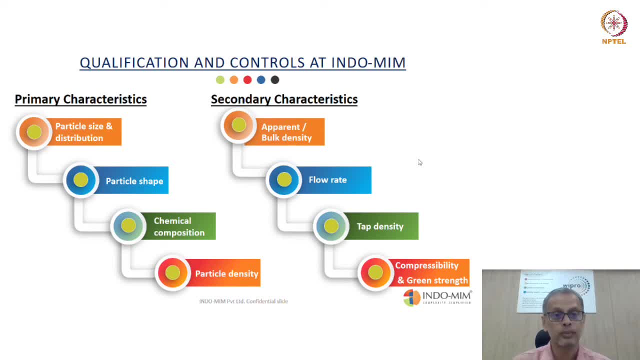 which are the minimum for these additive manufacturing folks to be able to use this powder and have lower failed print rates. Now what we are doing at Indomim is that we are fine tuning our process design. we are continuously iterating the process and having better controls so as to have all these particle shapes and distribution. 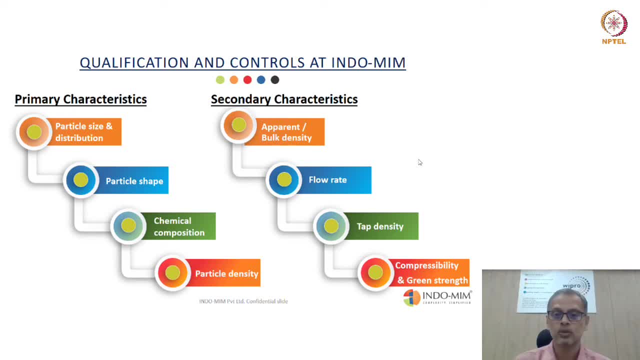 particle density that enables us to have mainly better tap density and flow rate. So flow rate is something which is an important secondary characteristic that directly affects the printing- the printer, I would say- and the in-house process capability measures that we have adopted. that is something which is helping us bring. 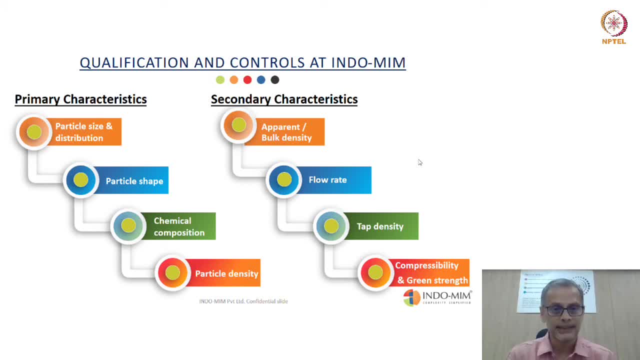 a better control in terms of powder consistency. I have also included in the presentation some of the control charts, which will have you proof of. the pudding is an eating kind of concept whereby you are able to see what kind of controls are actually being given out at Indomim, batch after batch. 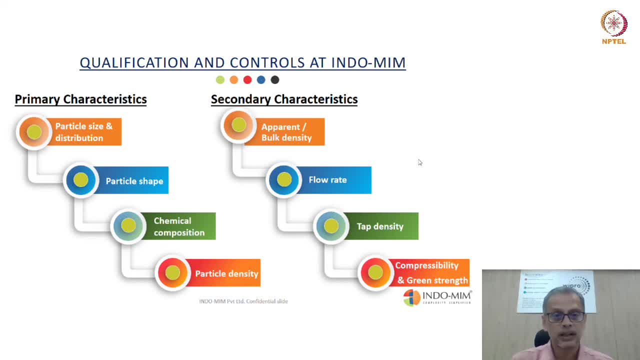 The particle size, distribution and morphology indirectly controls the apparent density and flow rate, as I was mentioning earlier. So just to kind of give you a kind of thumb rule. so if there is a good powder, what would happen is you pick up like 50 grams of powder, pass it through an orifice of, say, 1 inch. it should take. 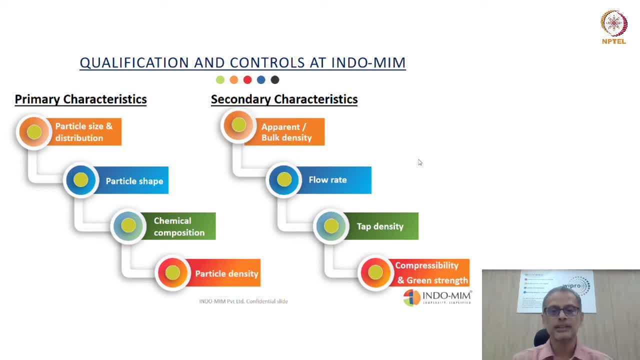 less than 20 seconds to flow. So this is one of the easiest or benchmark kind of method by which you are able to control the density and flow rate. So this is one of the easiest or benchmark kind of method by which you are able to. 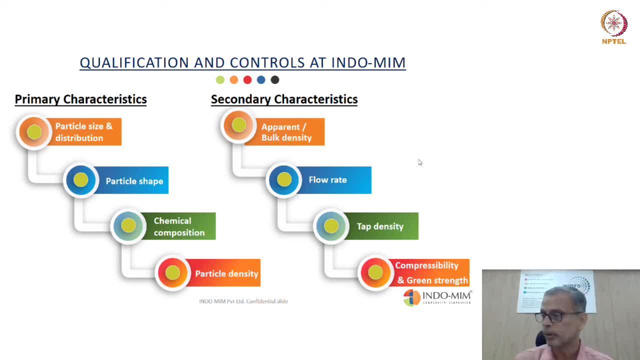 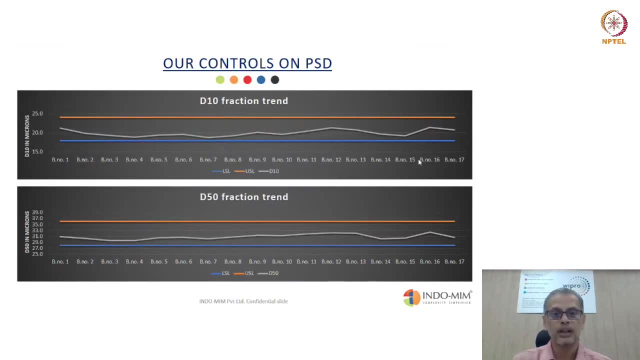 understand if the flow rate of the powder is good and if it is going to be helpful for the printing platform. So I was mentioning about these controls. So here are some of the particle size distribution control charts. In the upper chart you see D10 in microns and what you are seeing. 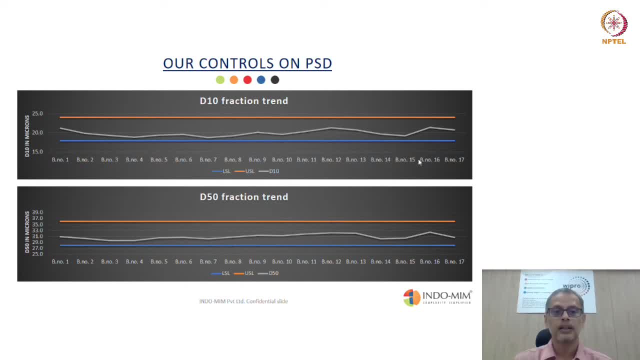 there is the blue one, which is the lower specification limit, the orange one is the upper specification limit and at the center is the D10- D10 control on particle size distribution starting from batch number 1 to batch number 17.. So what is controlled at INDO-MIM in terms of the process parameters is what is reflecting. 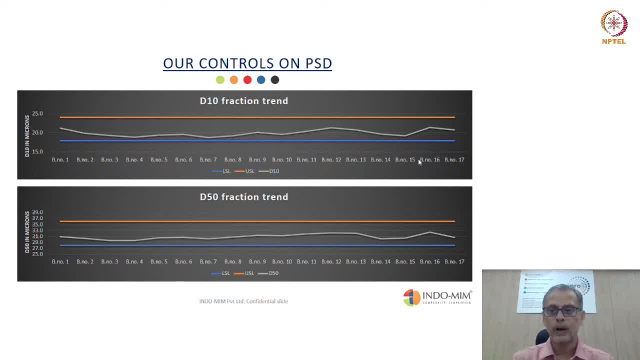 here in terms of result So well within the upper and lower specification limit. same thing you can see in the D50 fraction trend. again, the blue is lower specification limit, orange is the upper specification limit and the line as you can see, or trend as you can see, from batch 1 to batch 17,. we have just taken 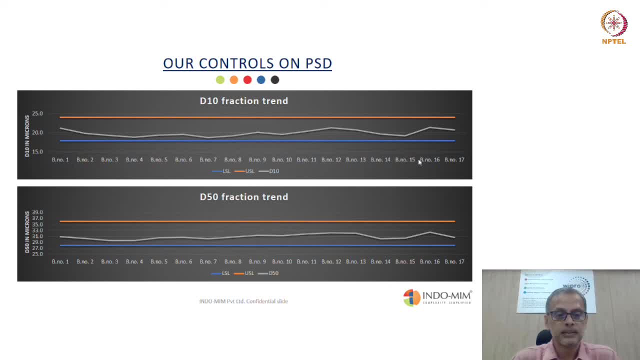 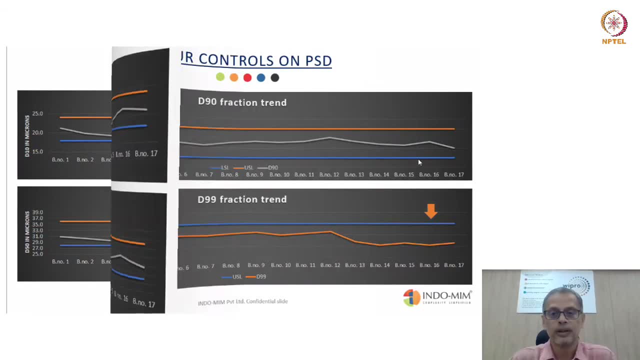 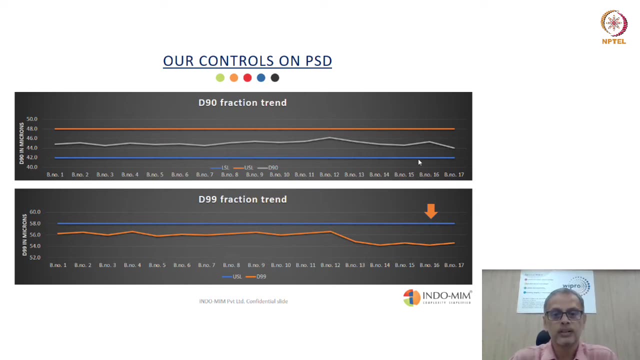 some example here that shows you that the output is very much in control within the upper and the lower limit. Here you have the controls on PSD for D90 fraction trend. so again you can see, between the lower and upper specification limit D90 is pretty consistent, pretty low in terms. 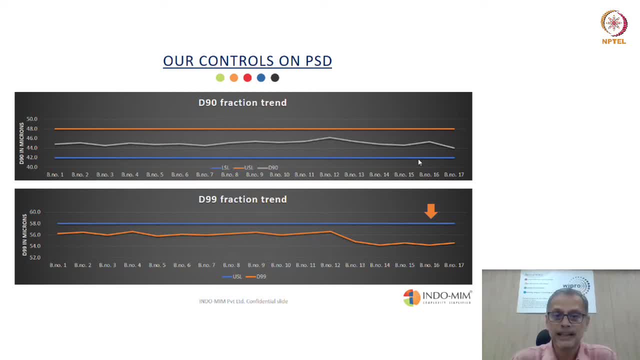 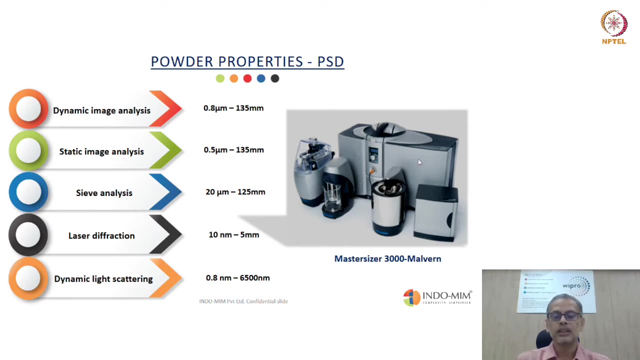 of the variation. and the last one is D99, where of course there is only upper specification limit and again, D99 is pretty much controlled. When we talk about powder particle size distribution trends, it is important to have these checked, the powder properties to be checked. 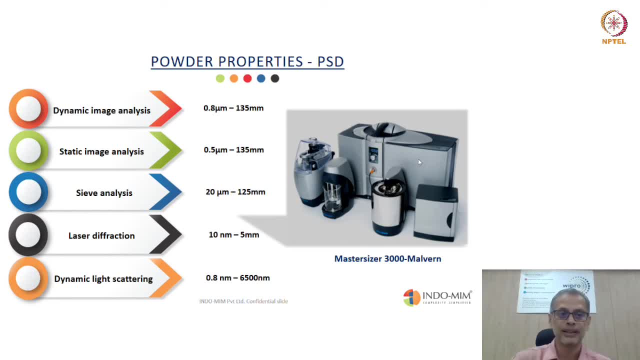 So these are some of the popular methods that are being used by the industry, Starting from dynamic image analysis, static image analysis, sieve analysis, laser diffraction and dynamic light scattering. So you can see on the right side. against each of these methods, we have also given 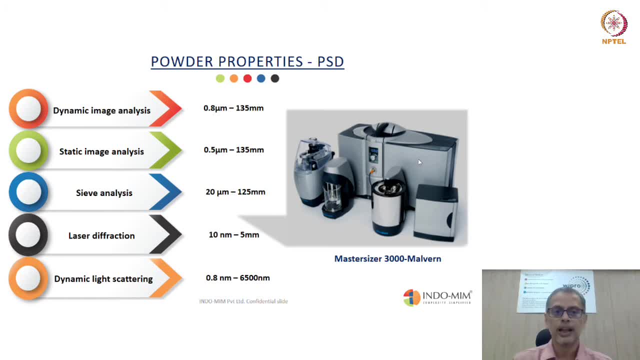 the range for this particle size distribution. for instance, for dynamic image analysis it is 0.8 microns to 135 microns. for laser diffraction it is about 10 nanometers to 5 mm. I mean, we at Indomim, of course, use laser diffraction. 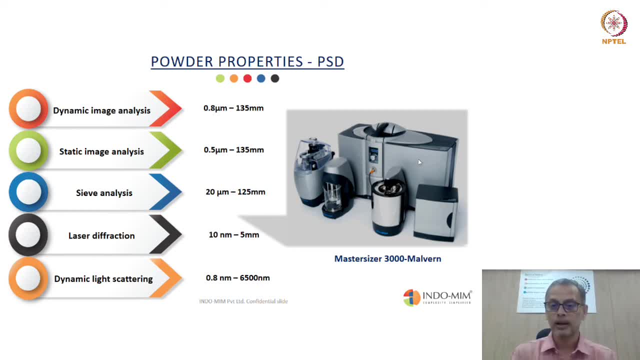 On the right side you can see the master sizer 3000 malvern. that is the instrument that we use. Of course we control from about 1 micron, starting from 1 micron upwards, using this laser diffraction method. But just out of academic perspective I thought we should include these different methodologies. 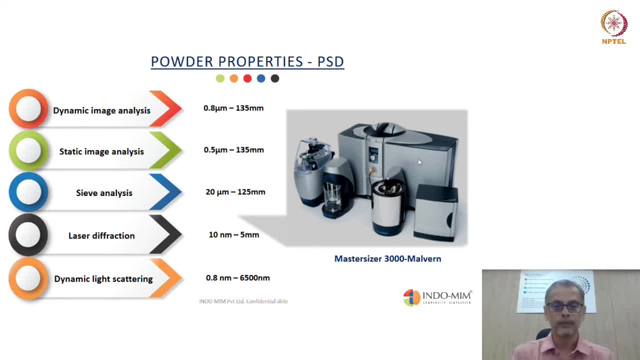 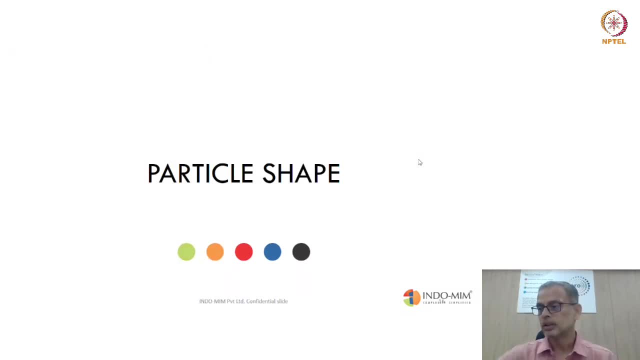 as well as the range that they can qualify or that they can check. So, having talked about the particle size distribution, particle size distribution or the methodologies to check them for outer properties and all, I think it is time for us to switch over the gears to particle shape. 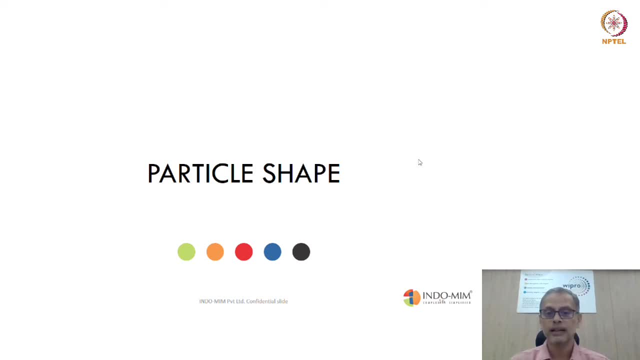 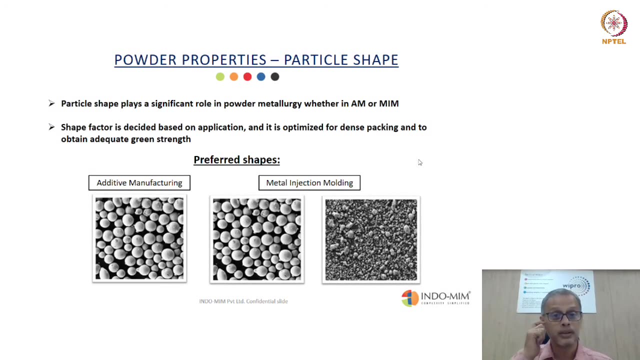 This is another important parameter that needs to be controlled when we come to additive manufacturing, and what does particle shape play in terms of role? So it has a very significant role in powder metallurgy, whether it is additive manufacturing or metal injection, molding, And shape is basically decided based on the application. If you remember early on, 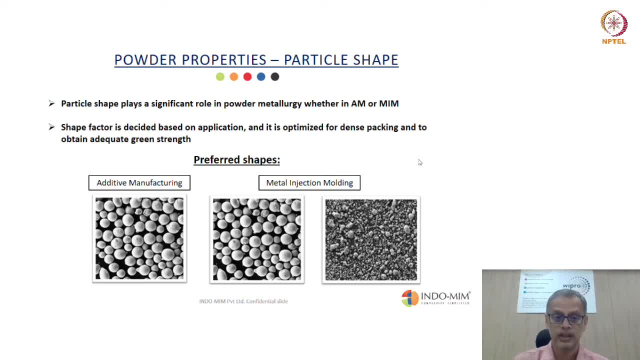 I just mentioned briefly that additive manufacturing needs spherical shape for having a better printing quality, whereas metal injection molding, wherein you mix the powders along with the binders and you need something called green strength. there you need a very good combination of irregular shape as well as the 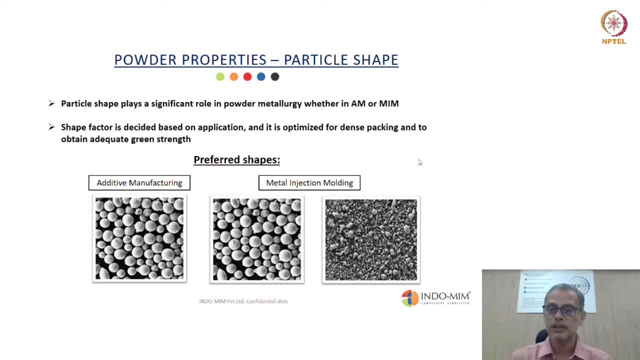 spherical shape. So the particle shape is going to be one of the main parameters, I would say, which is going to affect the process And in case of metal injection molding, the way it would be optimized is that it would enable dense packing to be done by having this. 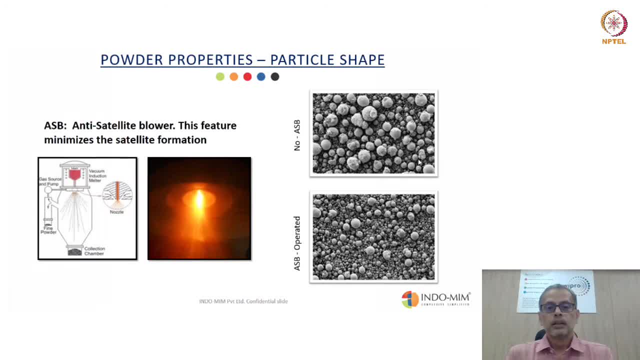 kind of combination Powder properties. again now, focusing on this ASB, that is a feature that Indomimum has jointly developed with our supplier. so anti-satellite blower. So what does this mean? This basically means that it is a feature that minimizes the satellite. 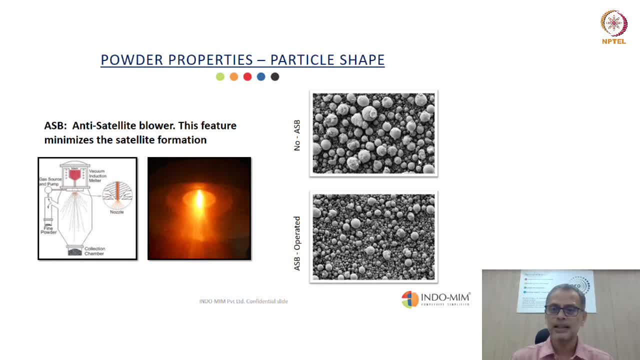 formation. Now, what is the satellite formation? As the word says, it is basically small particles which are kind of clung onto the large particles. So this is what is called satellite. So obviously you would be able to visualize that these small particles which are clung, 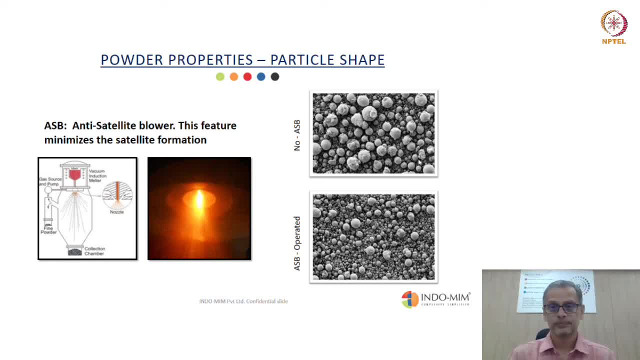 on to the large particles they would act as friction. So because of friction, what would happen is that it would cause it would become a deterrent to the flowability during the printing. So anti-satellite blower is a feature available in the process manufacturing process. that 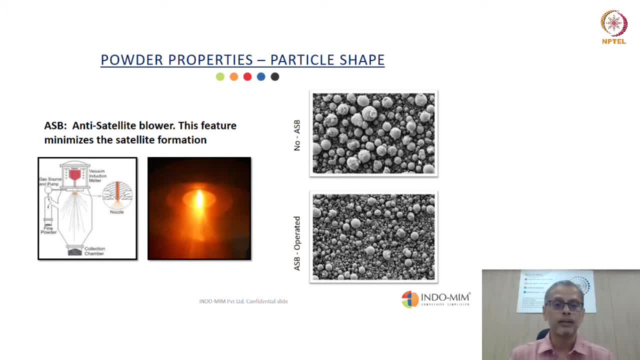 allows you to make the printing quality better. So you would not have friction on these smaller particles that are clung on to the major particles, and that is how you would have a better flow rate and hence a better printing quality. So the properties that are going to be affected in ASB anti-satellite blower kind of powder. 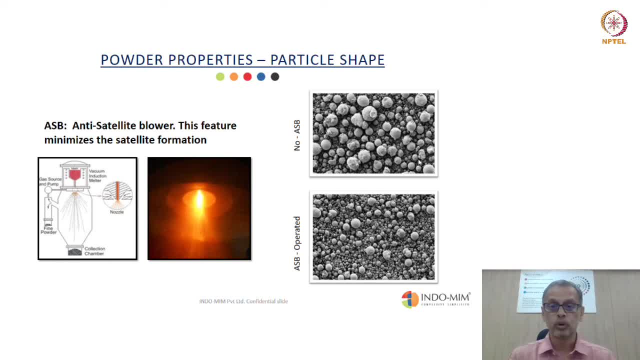 are going to be superior as compared to the no-ASB type. On the right side in this screen you can see on the top we have given a micrograph of no-ASB and on the bottom you can see a micrograph of ASB operated powder output. 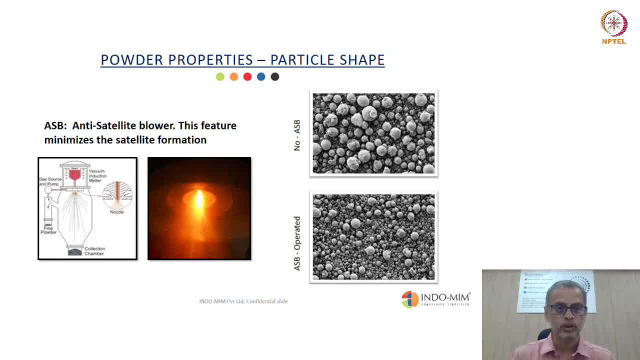 And the schematic of this ASB anti-satellite blower is shown on the left side. We have also taken a small photograph of the actual anti-satellite blower happening inside the atomization process, Just to make you understand What exactly is this particular feature. 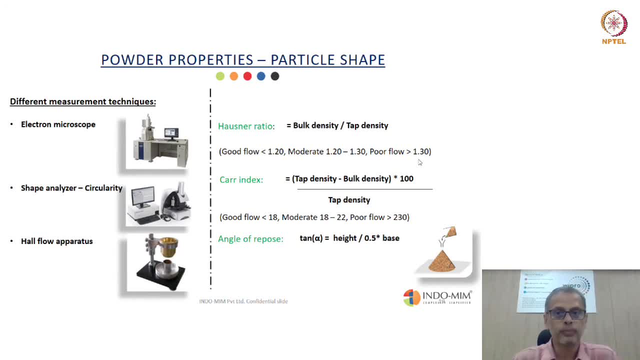 Coming to different measurement techniques. when we talk about the particle shape, electron microscope, shape analyzer for circularity and Hall flow apparatus for checking the flow. These are the three different measurement techniques that have been used: Hosner ratio and Carr index. I am sure most of you would be familiar by these parameters. 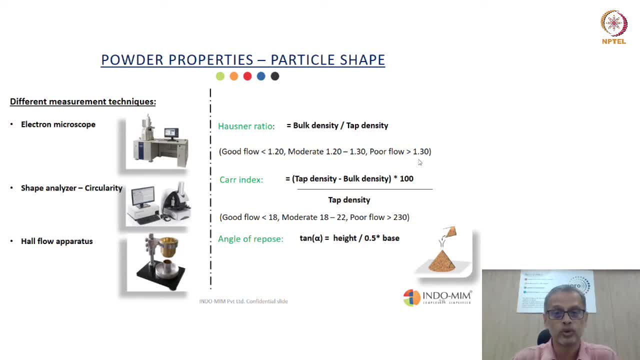 and this is something which are used- Which are the parameters that are used to basically designate the flowability of the powder. So good flow would be less than 1.2 Hosner ratio, moderate would be 1.2 to 1.3, and of 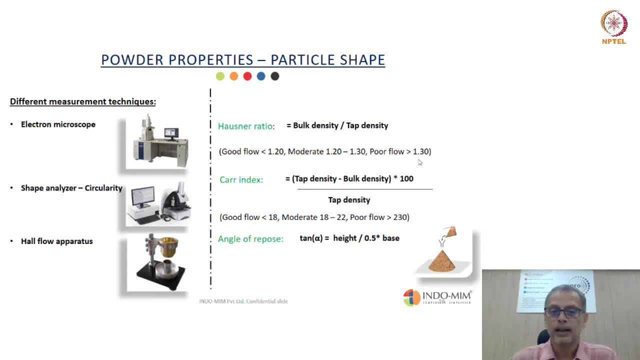 course, poor flow would be more than 1.3.. Again, on the Carr index, you would have good flow less than 18, moderate would be 18 to 22 and poor flow would be more than 23.. I am sorry for the small typo there. 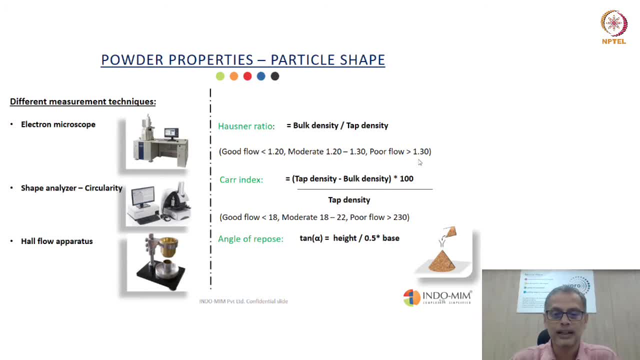 Coming to angle of repose: This is another thing. This is another thing. This is another parameter that is being used for the particle shape. I hope everyone is able to follow this particular thing as of now, and we will try to go to little. 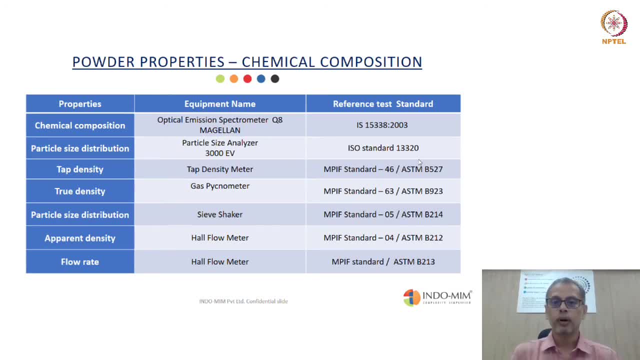 more details as we go into the next slides: Powder properties- chemical composition. so this is the slide which gives you details about the equipment that we are using for checking the particle size distribution or checking the tap density For true density, as well as the particle size distribution and apparent density. 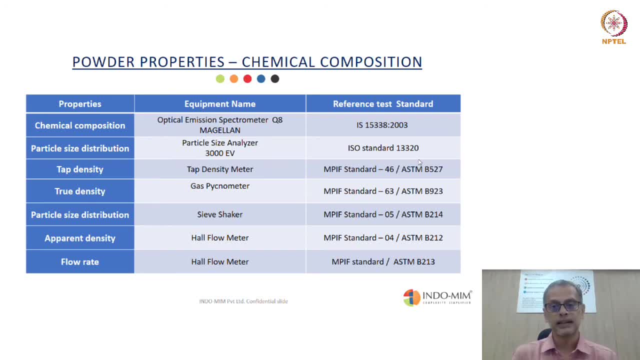 So these are the instruments that we are using and the reference test standards are given there. So, as you know, that MPIF- Metal Powder Industries Federation- that has a standard and, of course, aligning with ASTM and these ASTM and MPIF standard is something which we are using as. 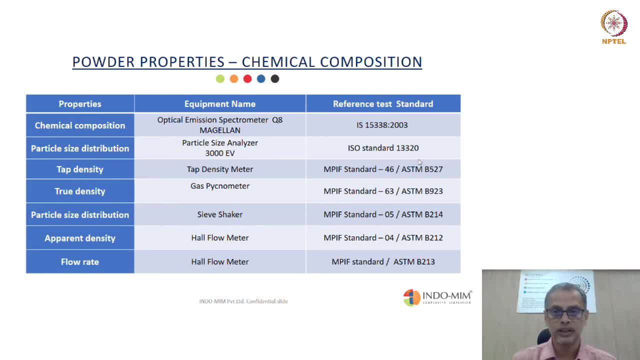 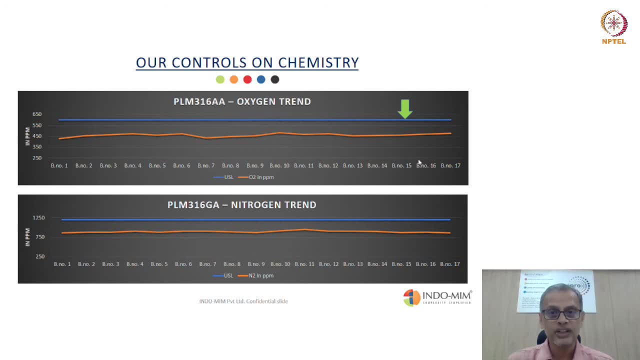 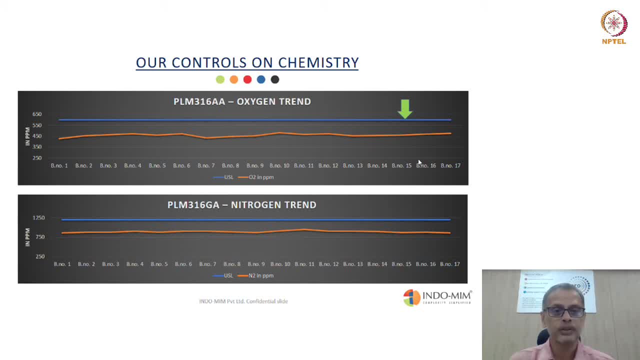 on chemistry. So these are the results in ppm, as you can see, and we are giving the O2 in ppm on the top chart and the bottom chart shows you the nitrogen in ppm. So very good controls on the O2 and nitrogen. 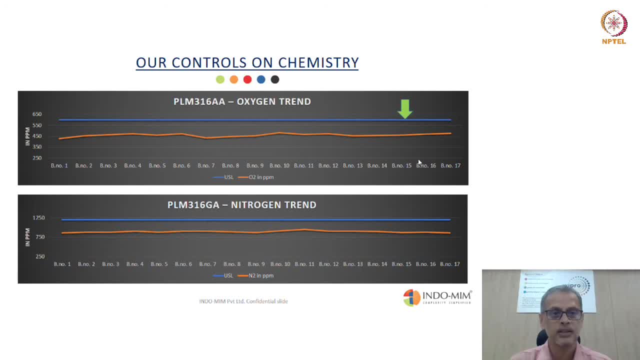 and you have the upper specification limits for both oxygen and nitrogen and at Indomim we are able to sufficiently control these well below the upper specification limit. I mean, needless to say, the lower the better. but again, if you want to have a better control, 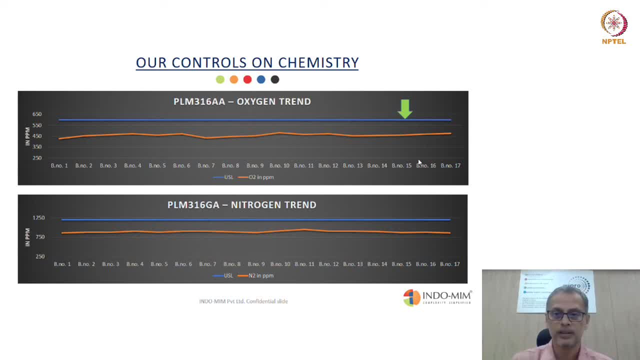 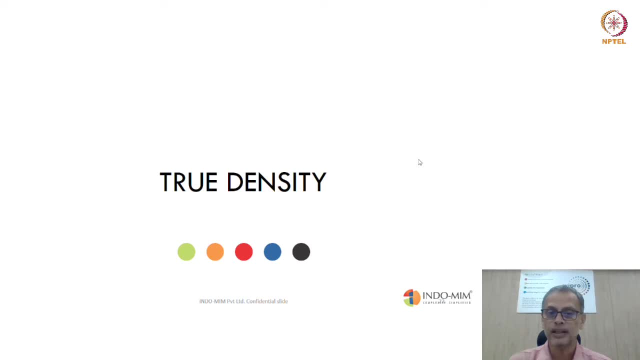 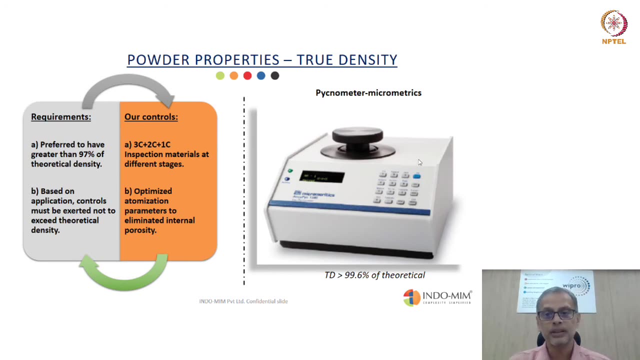 on oxygen and nitrogen. certainly you need to have higher manufacturing cost, Right. That brings us to the next important topic, that is true density, Right So, which is also a measure of the porosity present in the powder. So true density is something. 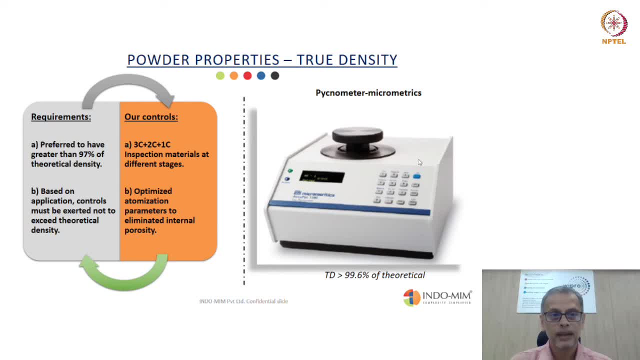 which we measure using an instrument called pyconometer, and on the left side you can see these requirements. Usually it is preferred to have greater than 97 percent of theoretical density, and for that what the controls that are available at Indomim are different. So for that we have to have greater than 97 percent of theoretical density. 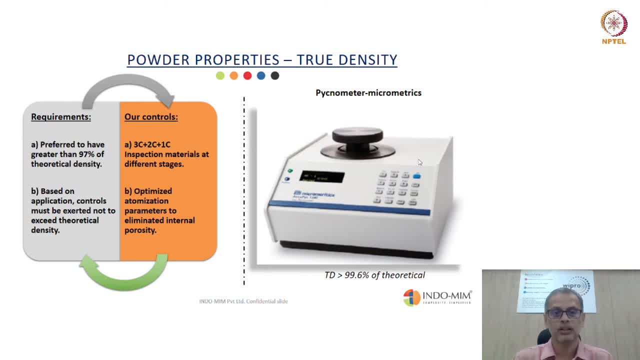 3C plus 2C plus 1C, that is the inspection of materials at different stages. So let me explain a bit about the 3C. So our raw metal supplier, they would, of course we would go and audit them or do a pre-qualification for them. that would be the first C. The second C would be the reports. 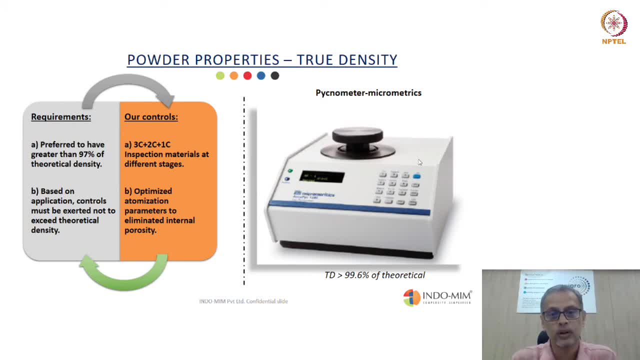 or the samples that they would send us for every melt that they are going to send it to us, Right? So we would have, we would maintain records for that. That is the second C, and the third C is the raw material inspection that we would do upon the arrival of powder. So if you recall when I was 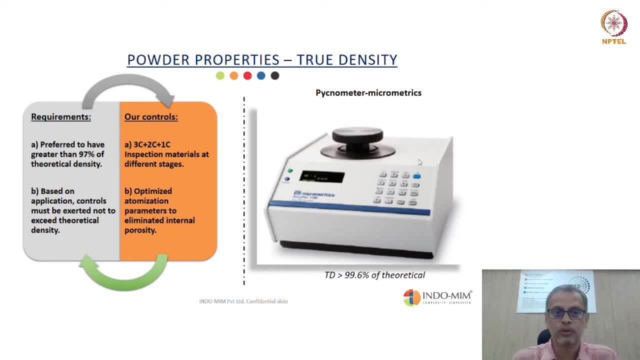 explaining the process flow for the powder manufacturing. I was showing you that the in-process inspection is something which happens at Indomim for every arriving batch Right. So that is the third C. Now, when we come to 2C, this is basically the process inspection that is being. 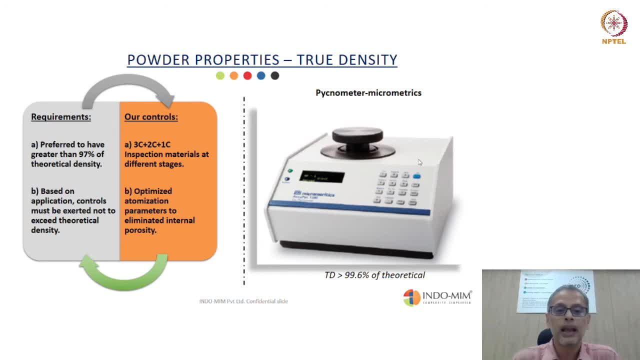 done in process inspection and the process inspection that is being done in process inspection, The final inspection that is being done. and 1C is the final inspection that is being done before the dispatch of the powder to our customer. So another requirement is that, based on the 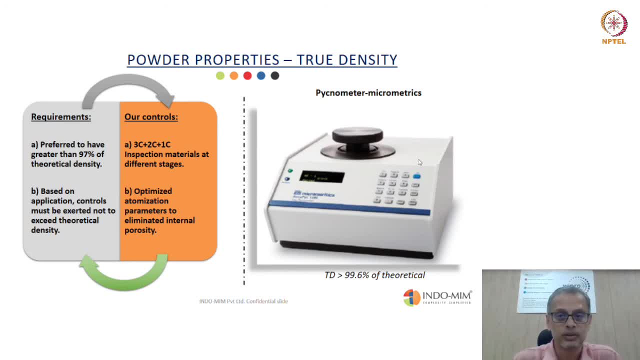 application, the controls must be exerted not to exceed the theoretical density. So this is one of the important parameter. So what we do is we optimize the atomization parameter to ensure that the internal porosity is eliminated Right To a large extent. So true, density, as I said, is a 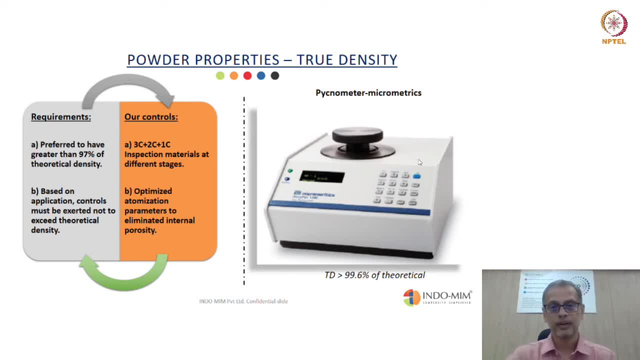 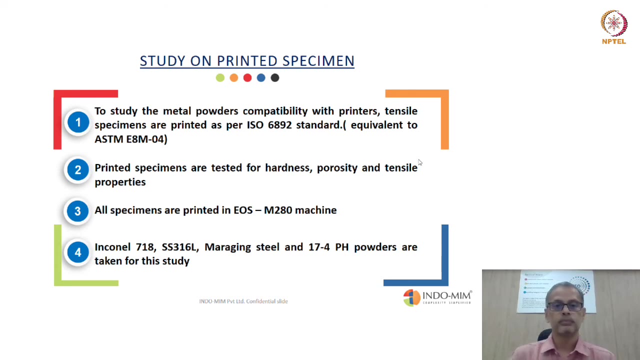 measure of how much porosity, internal porosity, is available. Every powder has certain internal porosity and for us to assess how much of this internal porosity is available, we check the true density using this pycnometer. Right Now, coming to the study on the printed specimen, what we do is we study the metal. 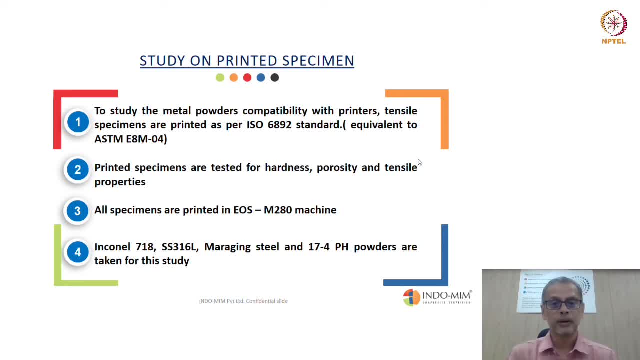 powders. compatibility with printers that tensile specimens are printed as per the ISO 6892 standard, which is, of course, equivalent to the ASTM standard given here. So, then, these printed specimens are tested for hardness, porosity and tensile properties. All the specimens are printed. 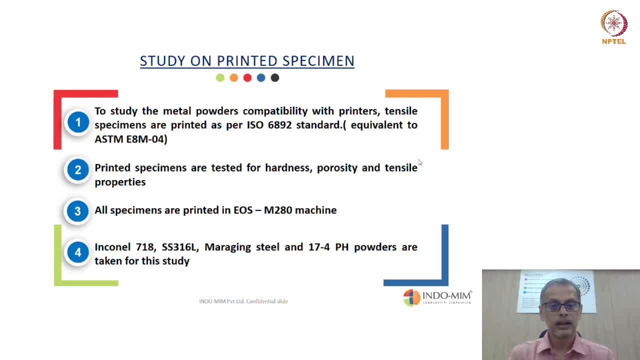 in US and our team has really taken good lead in having a wonderful collaboration with US, which is the world s largest company for making these printers. So we have identified a specific machine, M 280, on which all these printed specimens are tested, and this kind of collaboration between 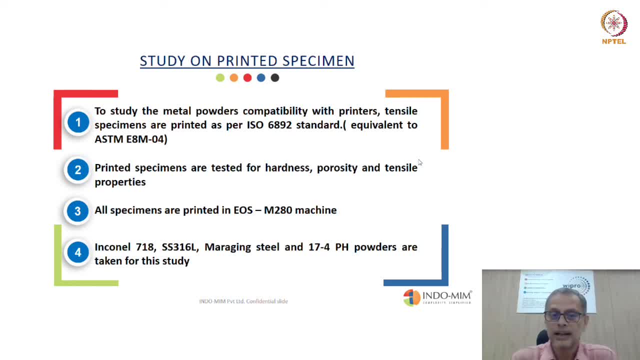 Indomem and US is something which is standardized. So we have the help of a few folks and we are is standardized and that is something which is followed for powder qualification process. This enables us to have a standardized thing. So what we have done is we have taken Inconel 718,. 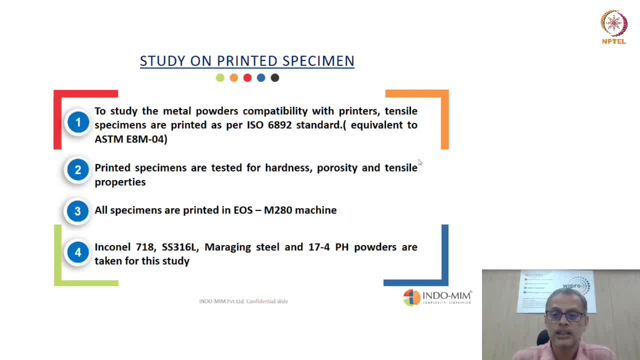 we have taken SS316L, we have taken Maraging Steel and 17-4 PH. These are the four powders that we have taken for study and we carried out these studies with the printer basically to assess how good are the mechanical properties compared to conventional processed materials and standard. 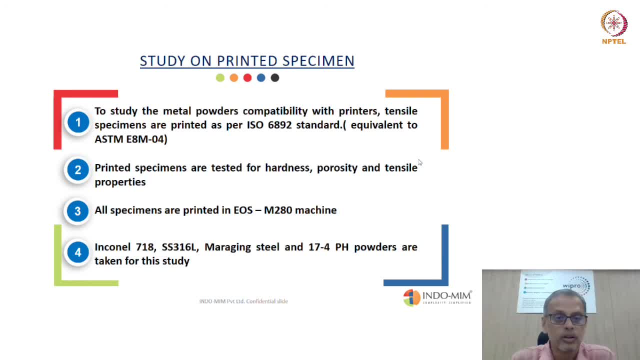 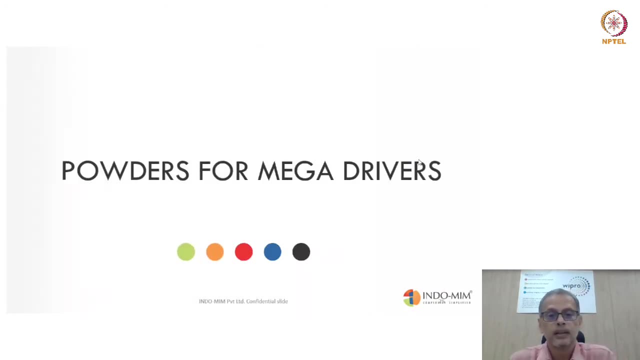 values of the printed specimens from the other manufacturers. So unless you benchmark, I am sure you would agree that it is very difficult for you to indicate your USP. So, powders for mega drivers, everything we have talked about, the powders we have talked. 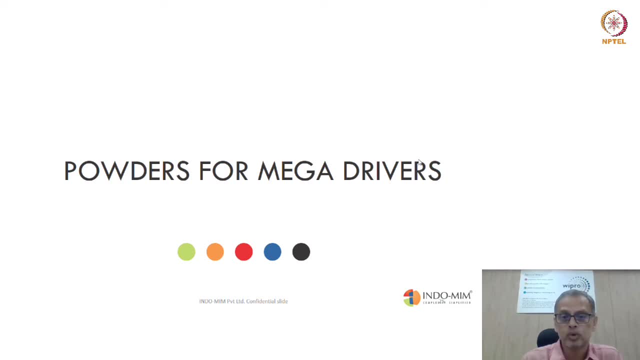 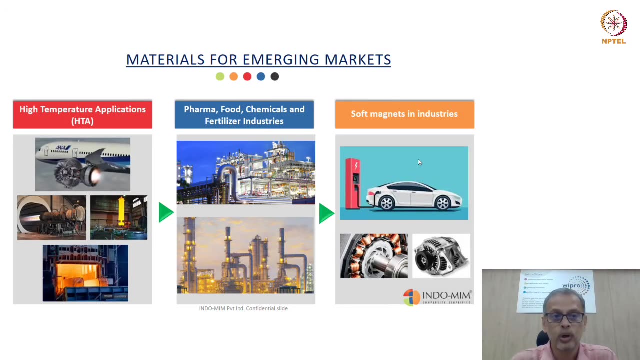 about the manufacturing properties. we have talked about the manufacturing properties process, but it is also important to identify or to correlate this powder production with respect to the industry. Of course, all of you are from academic background, but there are, I am sure, some people in the 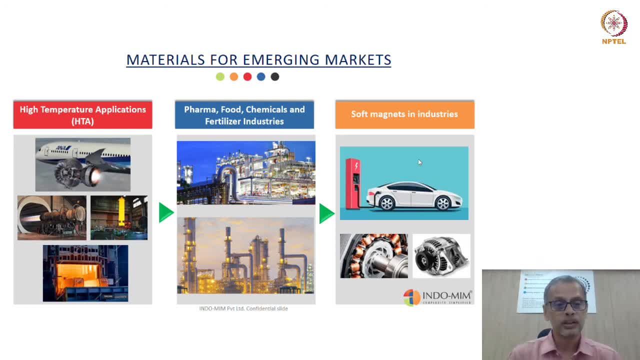 audience who are also from the industry side. so you would be certainly curious to know that. what are the materials for the emerging market? So what kind of applications are coming up in the coming years, and where exactly is the industry delving so as to help us, people like us who are powder manufacturers to be? 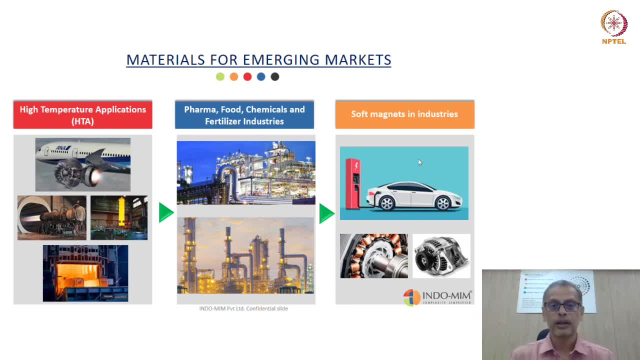 able to catch up with the upcoming requirements and thereby support. So when we come to high-temperature applications, these are the ones that you can see are clearly emerging. On the high-temperature applications, Aerospace, you know that is one of the areas that is certainly demanding for this. 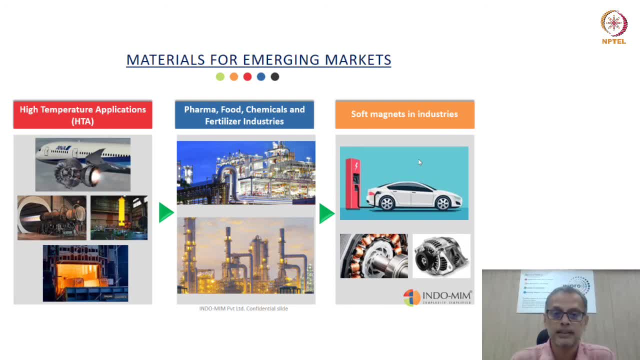 Coming to pharma, food chemicals and fertilizer industries, again, there are very, very specific and niche requirements that are helping us to identify these things and develop the specific powders And soft magnets I mean. EV, as you all know, is something which is an emerging application. 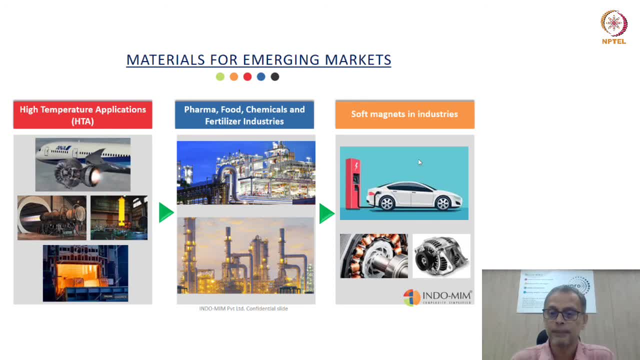 which is catching up very fast both on the two-wheeler as well as the four-wheeler side, And EV is demanding a lot of support from the powder manufacturers, And so we are doing a lot of activity for the EV as well. 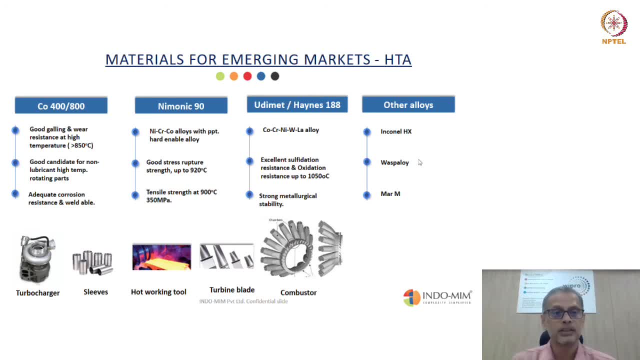 So let us go into all these specific market applications one by one. So here are the four major alloys that we have developed for applications from the HTA high-temperature applications, which spans across the industries of manufacturers like turbocharger manufacturers, like people who manufacture sleeves. 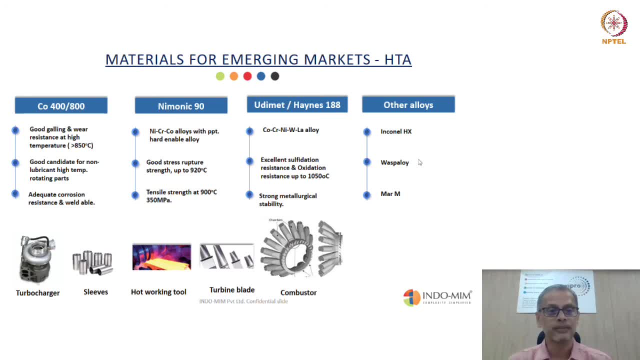 Hot working tool, turbine blade, combustor and these kind of applications. So when we come to cobalt 400 and 800, good galling and wear resistance at high temperatures is something which is required. more than 50 degree centigrade. 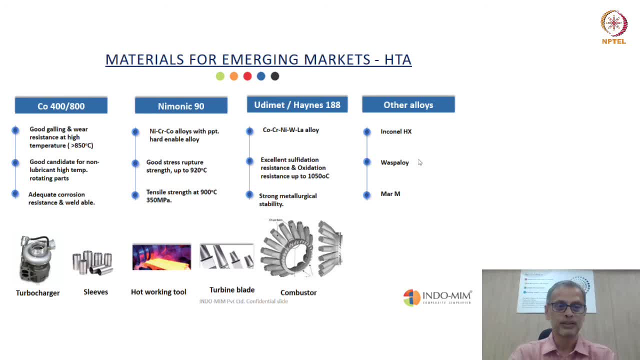 This powder is a good candidate for non-lubricant, high-temperature rotating parts, And adequate corrosion resistance and weldability is something which is important for this powder, which is one of the key characteristics When we come to nimonic 90.. 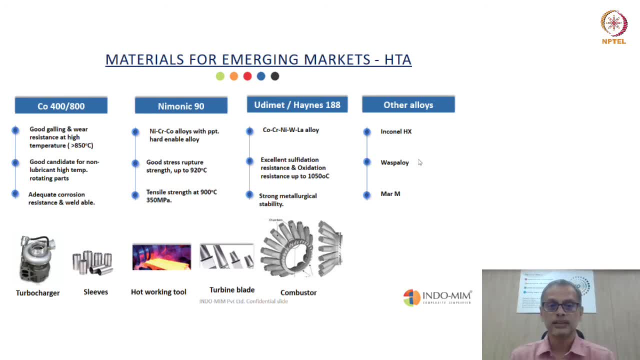 Nickel, chromium and cobalt alloys. these are something. this is something which is the hallmark of nimonic 90. It has a good stress rupture strength up to about 90 degree centigrade. So turbochargers are ones which are using these particular materials to a large extent. 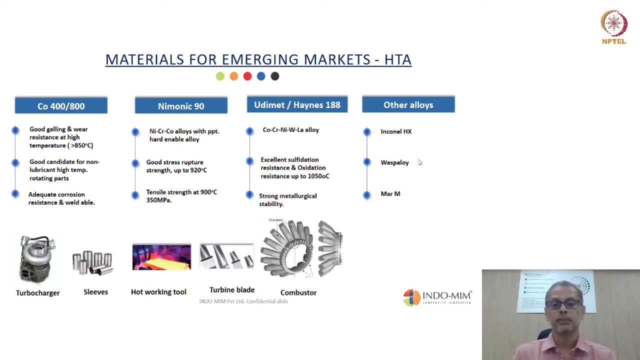 It has a tensile strength of about 350 megapascals at about 90 degree centigrade. So this is something which is very unique for nimonic 90.. Coming to UDIMATE, or Haines 188.. This is again a cobalt-chrome-nickel alloy. 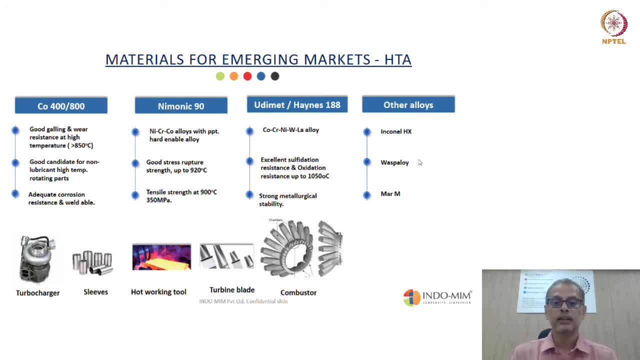 This is a tungsten alloy which has an excellent sulfidation and oxidation resistance up to about 1050 degree centigrade, And it has a very, very strong metallurgical stability. Some of the other alloys that we have been developing for these markets are Enconel HX. 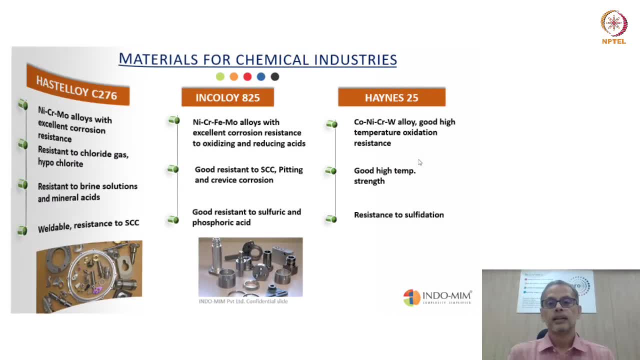 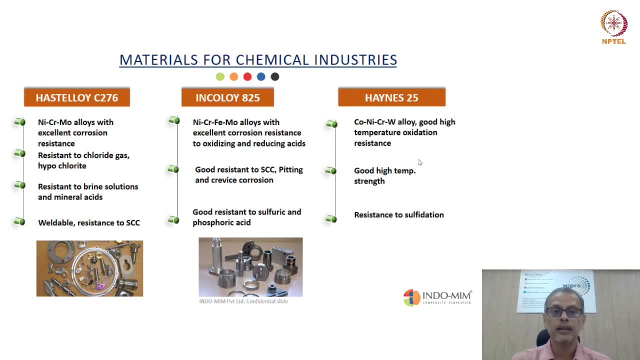 Baspaloy and Mar-M. Coming to chemical industries, or I would say also pharma industries, which can be covered in this category, The three main materials that we have been developing for these markets are Enconel, HX, Baspaloy and Mar-M. 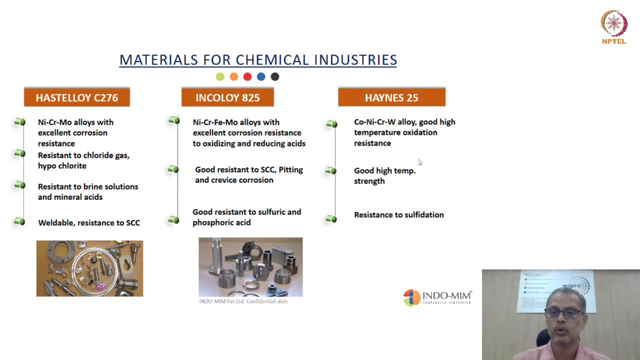 Some of the other materials that we are developing here is Hestaloys C26, Encloy 825 and Haines 25.. Nickel-chromium molybdenum alloys with excellent corrosion resistance is the hallmark for C276 of Hestaloys. 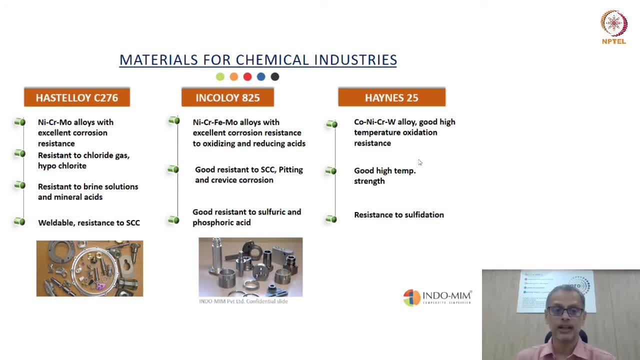 It is resistant to chloride gas and hypochlorite, So any application that demands these kind of resistance can definitely use this kind of material. It is also resistant to brine solutions and mineral adhesives And, of course, needless to say, it is weldable and resistant to SCC. 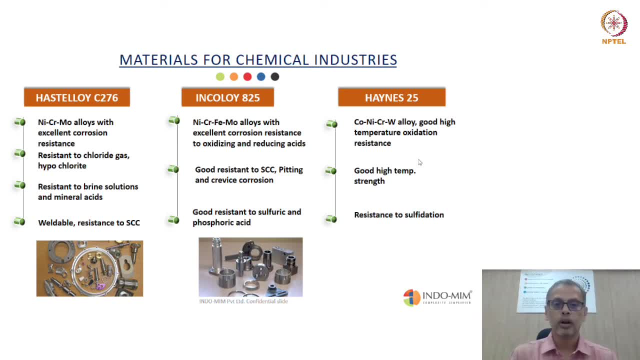 The second alloy is nickel-chromium-iron- molybdenum alloy. It again has excellent corrosion resistance to oxidizing and reducing acids. It has good resistance to SCC, pitting and crevice corrosion and also good resistance to sulfuric and phosphoric acid. 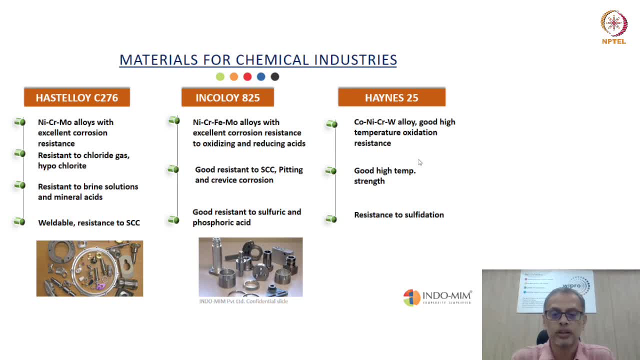 So we have also shown some of the images at the bottom of these specific materials. Haines 25 is a cobalt-nickel-chromium tungsten alloy with good high temperature oxidization. It has also excellent corrosion resistance to oxidizing and reducing acids. 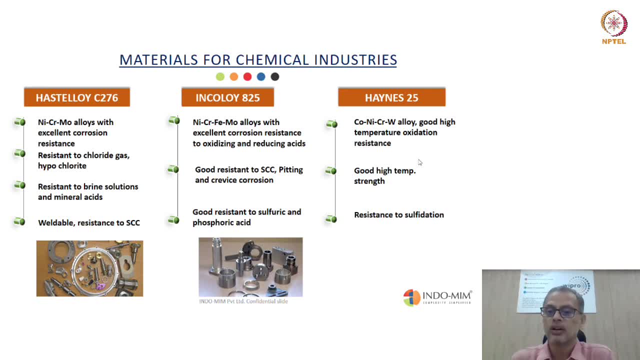 It has also excellent corrosion resistance to sodic acid. It has also excellent corrosion resistance to citric acid, temperature oxidation resistance, also good high temperature strength and resistance to sulfidation. So based on these properties for these specific materials, the industries can select. and there 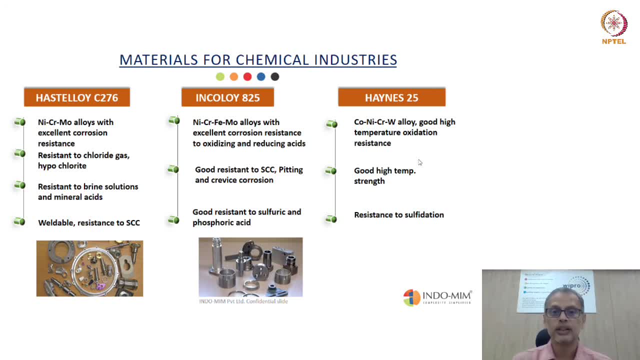 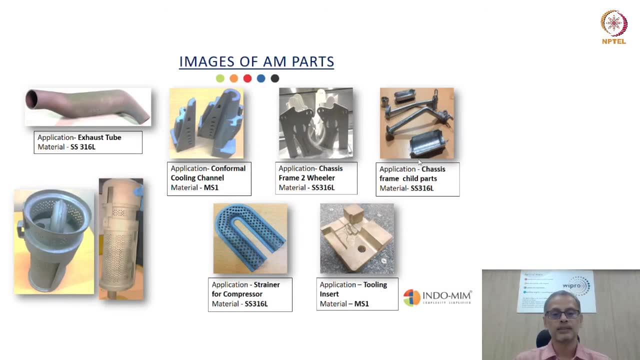 is a lot of support that Indomim engineers are providing to the industry in terms of understanding the requirements and tailoring our processes to get these kind of parts for the specific industry. Here are some of the images of additive manufacturing parts. I mean we have also thanks to our partner industry from the 3D printing who helped us. 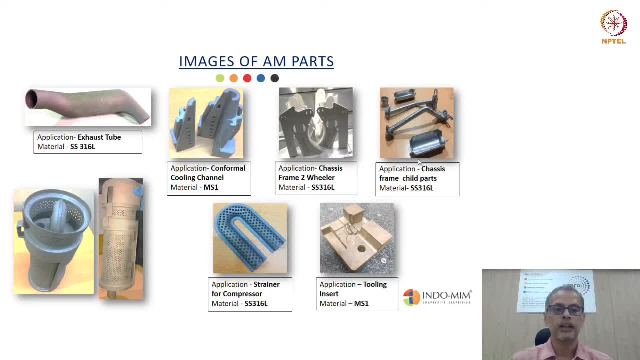 to get these images. courtesy. Application is exhaust tube, as you see at the top left, which is material of SS316L. There is another application of conformal cooling channel in material MS1. that has been done using 3D printing. The third one you can see in the sequence is chassis frame for a two-wheeler. 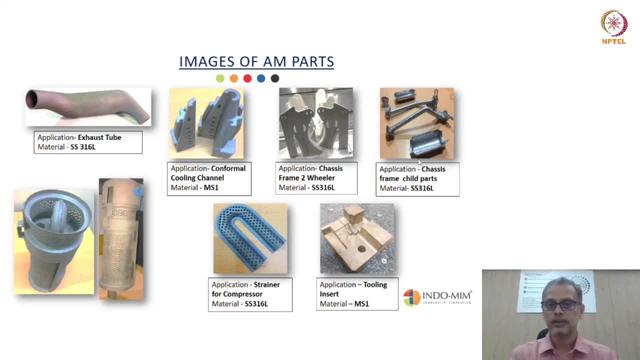 It is a pretty large component in 316 that we have That. this we have helped to additive manufacture. through additive manufacturing There are other chassis, frame, child parts which are made on the fourth one, And then you have strainer for compressor and tooling insert. I mean that this particular 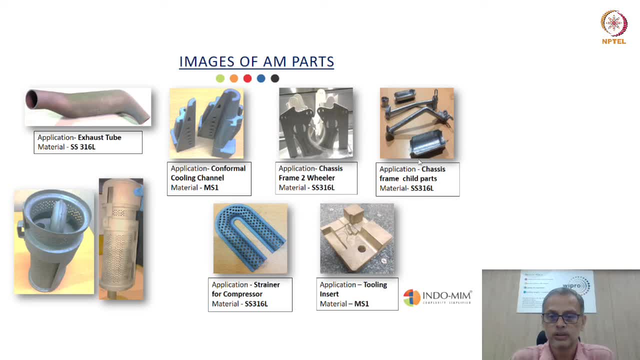 additive manufacturing company is making for us, for our own captive consumption. So the reason I thought we should include these images of additive manufacturing parts are: these are the kind of parts that are used by the powder that we are supplying. They are printed by the powder. 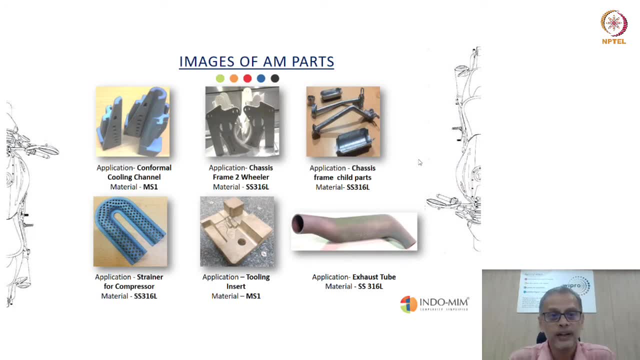 Here are some more classified images. you know, as per the industry, These are the images for, for instance, for two-wheeler segment. as you can see from the end images of representative images of motorcycles that these are parts which go for specific. 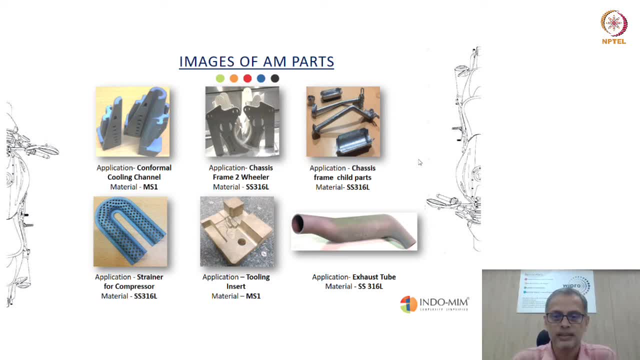 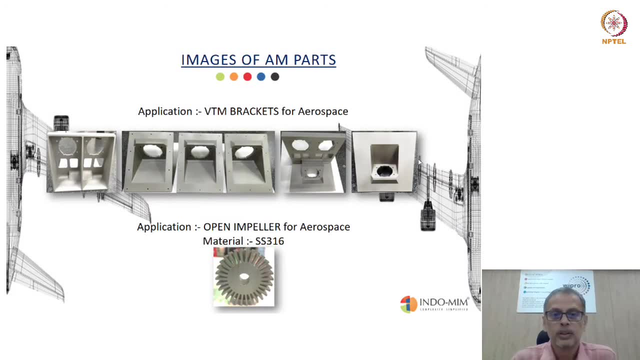 to two-wheeler industry and again spanning across various materials and spanning across various shapes. Here are the applications of aerospace: We are making powders which are being used to make VTM brackets, as well as the impeller, you know, open impellers. 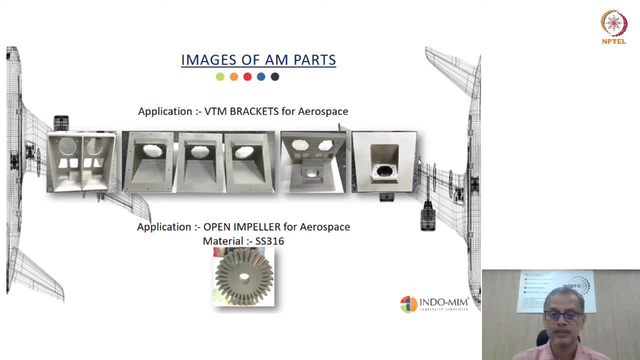 As you can see, the image of open impeller material is SS316.. The shape is pretty complex, right, And making such kind of impellers through conventional processes is going to be very, very tough. Using machining, you can take ages and hours and days to make these kind of products. 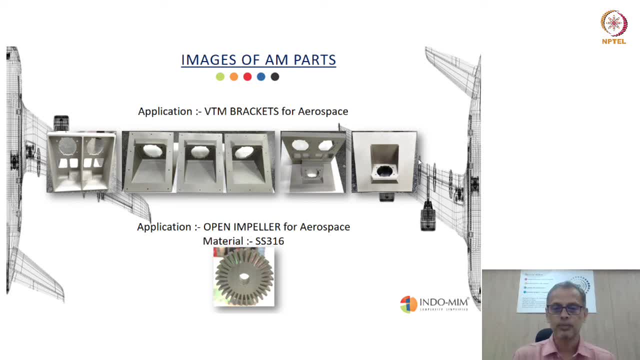 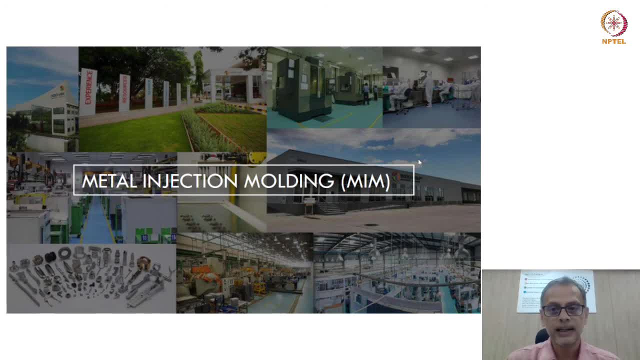 Having talked about additive manufacturing in detail, I think time has come for me to also touch upon metal injection molding. That is one of the process which is at the core of Endomim. As I said, we are the worlds largest company engaged into making this metal injection molding. 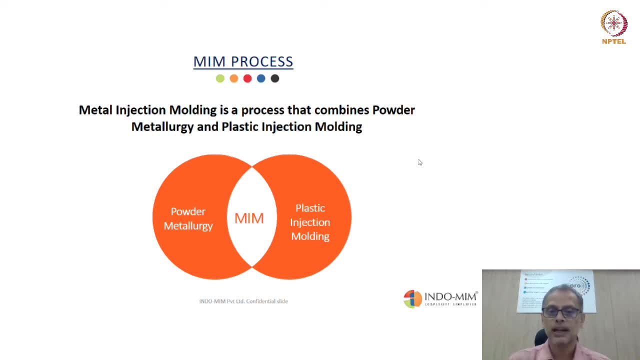 process Friends, metal injection molding is a process that has the best of both worlds: one of the world called powder metallurgy and another world called plastic injection molding. So what we have done, what this process has done, metal injection molding, is it has picked. 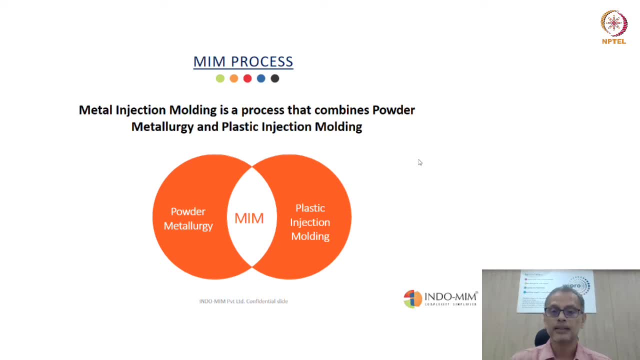 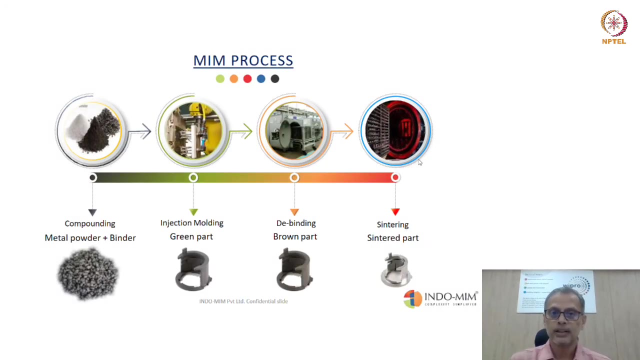 up the alloying benefits from powder metallurgy and it has picked up the shape making benefits or shape making capability feature of plastic injection molding and it has evolved as a process that has best of both these worlds. So MIM as we call it as an abbreviation. MIM is a four-step process starting from compounding. 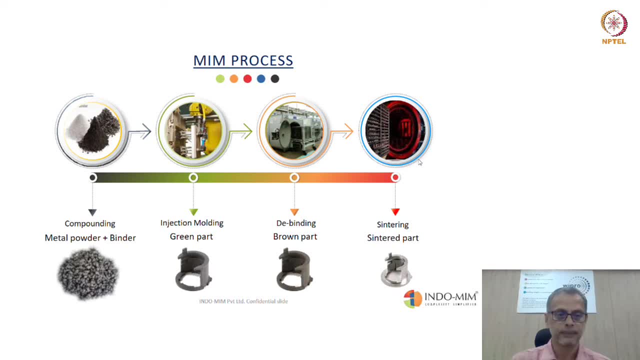 injection, molding, followed by debinding and sintering. So what is compounding? Compounding is basically a process where we mix the metal powders that are produced by atomization process- gas and water atomization- and these are mixed with binders. 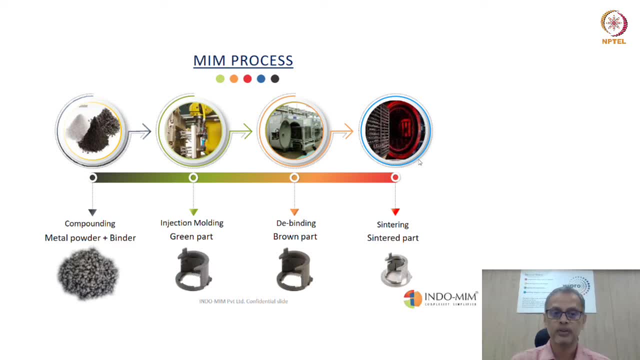 So we have four different components of binders that we use to mix along with the metal powders and we mix them with the metal powders And then feedstock is made. So in the image you see, white color is the binder representative binder- black color. 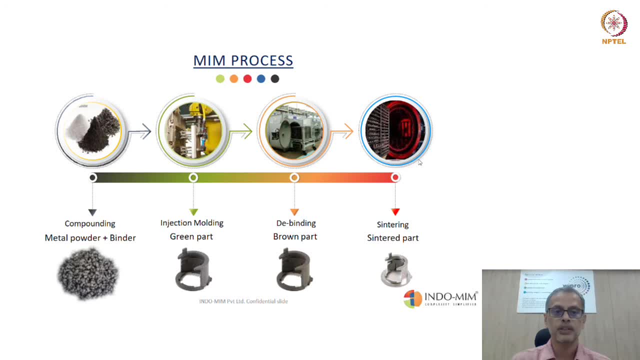 is the powder, and on the farther end you see the feedstock, which is very similar to plastic injection molding granules, just that here it has a mixture of metal powders and binders, So the feedstock is something which is injected into the mold at the injection molding stage. 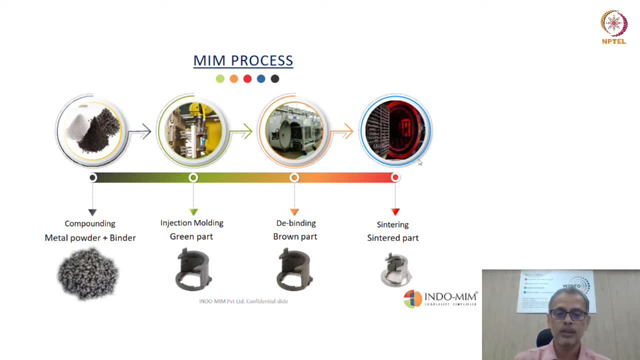 and that is something which gives us the green part. So you can see an image of the green part Now. this green part has the entire shape or contour of the part that you, as a customer, intend to have. However, the part is oversized. 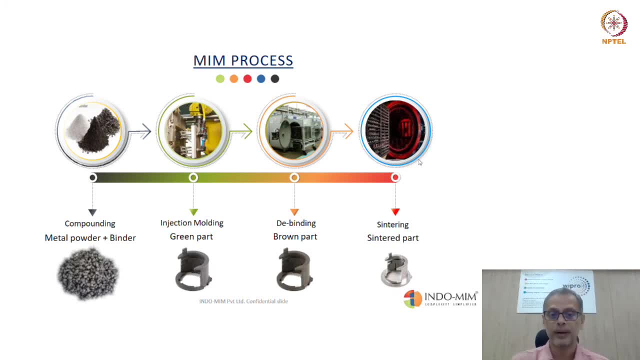 The reason I say oversized is it has content of binder in it. So what would happen necessarily in the next two stages is that we would have debinding and sintering to the removal of binders. So the first, So the major component of binder, which is basically called the primary binder, is removed. 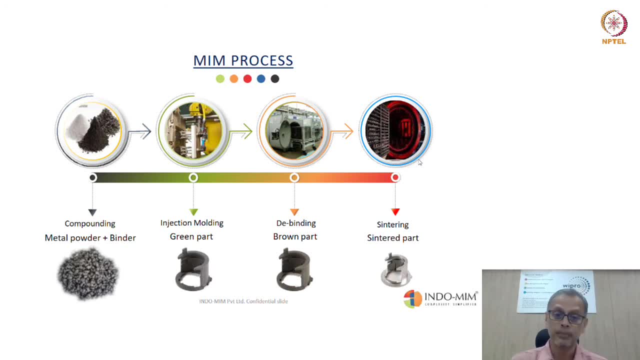 at the solventee binding stage and at this stage we call the output as brown part and the remaining component binder. secondary component binder is still with the component holding the metal particles together. At this stage we put the part to sintering. 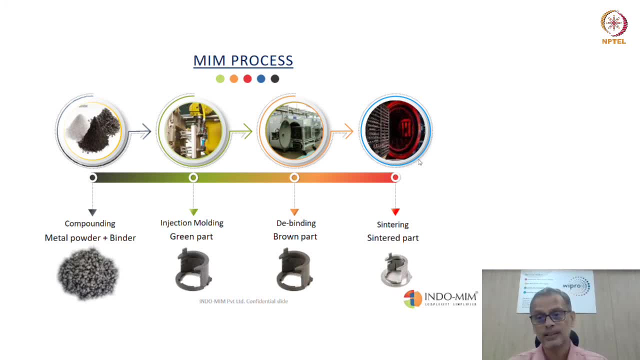 Now, inside the sintering furnace, we have two types of furnaces: vacuum furnace as well as continuous furnace. Here, the first stage of the process is called thermal dividing. This is the process wherein we allow the secondary binders to evaporate and, with the completion, 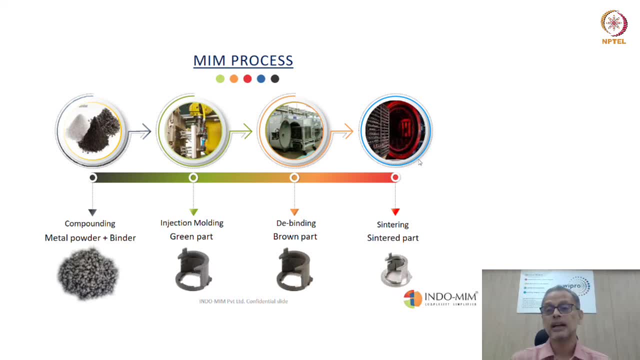 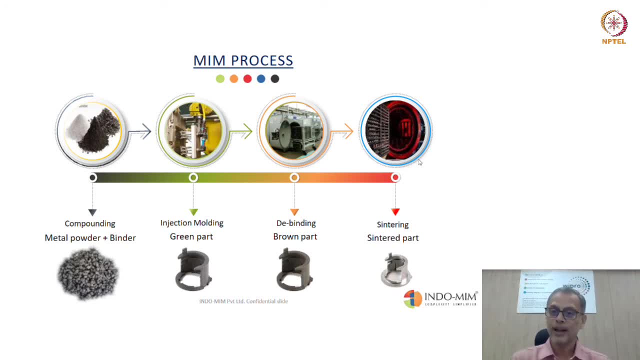 So this is indicative of the 20 percent shrinkage. So this is indicative of the 20 percent shrinkage. So why does 20 percent shrinkage happen? The intermolecular diffusion that happens inside the sintering furnace is the main reason. 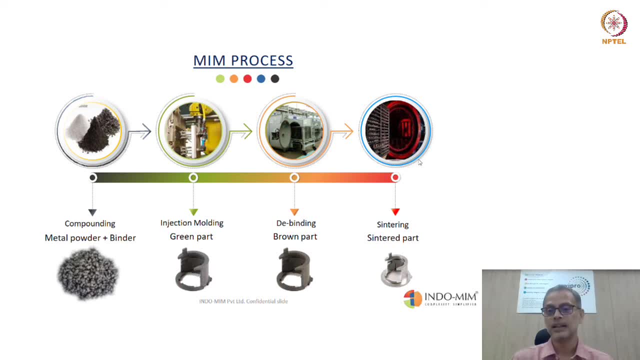 why 20 percent shrinkage occurs, and this gives the density to the process. So what we say usually is that metal injection molding is a process that enables you to get complex shaped parts with full strength, which means there is no compromise in strength, but still you are having to make sure that the parts are in the correct shape. 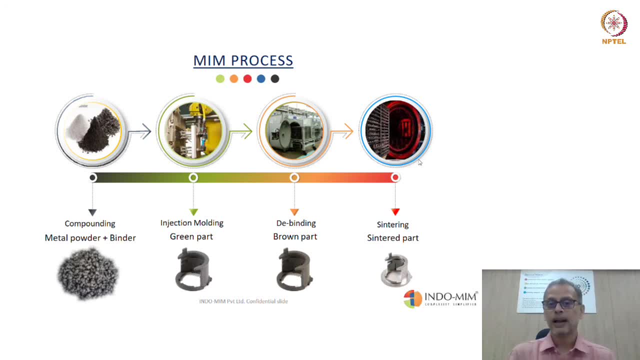 So this is indicative of the 20 percent shrinkage. a metal forming process. produce it. you are not doing metal cutting and in simple things, if I can tell you, metal cutting is something which enables production of bur. So MIM process is a metal. 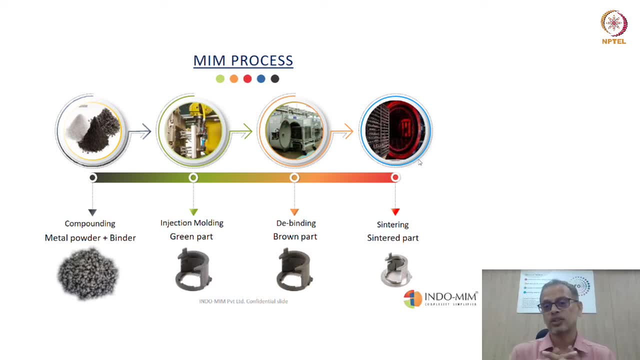 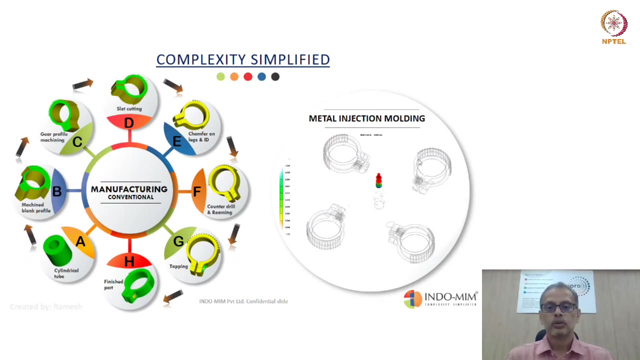 forming process that eliminates the production of bur itself. So that is one of the very, very important deterrent that any manufacturing shop flow fellow would kind of be worried about. that is something which is completely absent here in metal injection molding, going to the way this process is designed. So here is an example. I mean 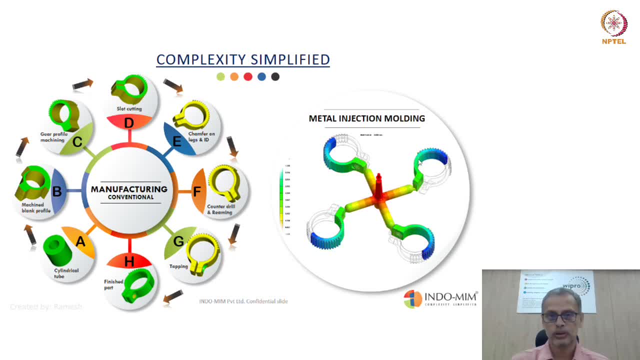 for you to understand what kind of complexity are we talking about? In the MIM, the tagline is complexity simplified. So when we say complexity simplified, what kind of complexity are we talking about? So on the left side you can see it is a 8 step process for a component that you see of 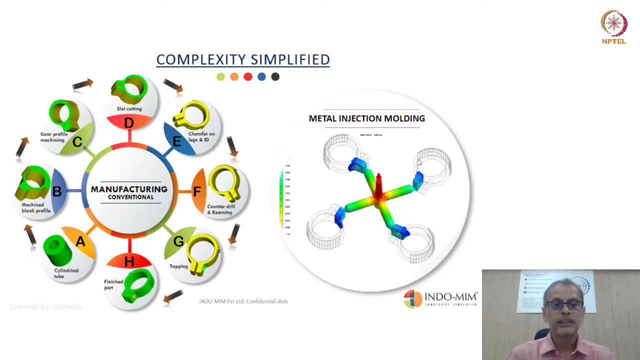 course on the last H stage. that is the finished part. So this is basically a steel part you can blew in to making some chic can porous4 system and the rest is for the use. what is the process that is being used for an automotive application for fuel? 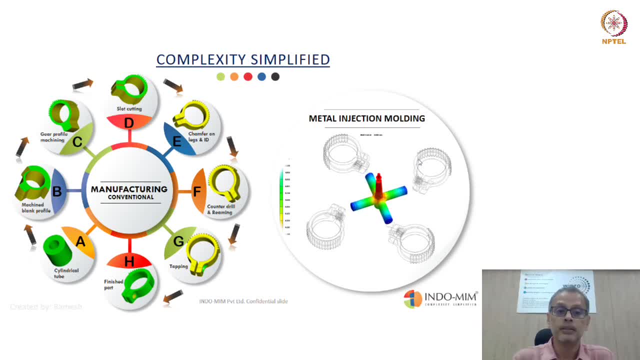 control or fuel flow control, I would say So, starting from A to H are the specific processes, the legs and ID, followed by counter drilling and reaming, tapping and finally the finished part. Now to have all these features on the component, if you can see on the right side. 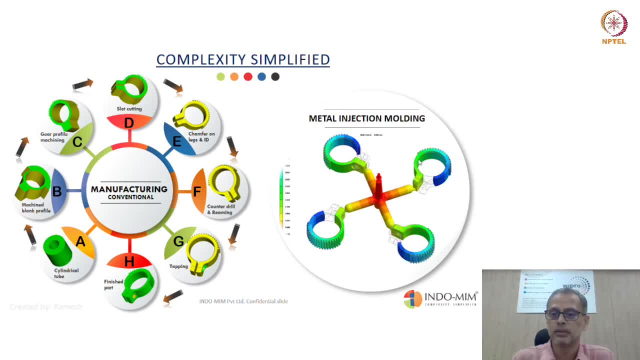 metal injection molding just uses a very simple molding step which gives the entire profile, entire form, and here you have a single drop that is shown, single drop of the hot runner that is shown. We have a 8 cavity or 16 cavity mold for this particular component and the beauty is that. 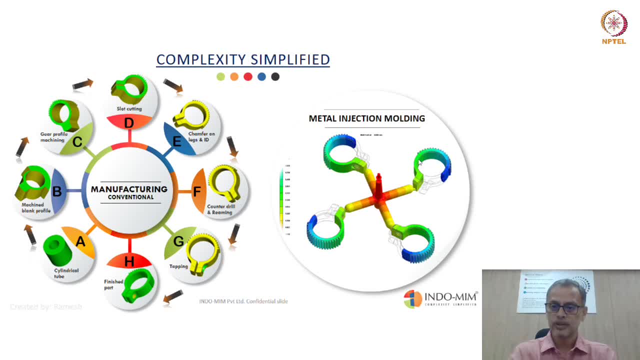 the entire feedstock flows inside the mold, which has been designed in manufacturing ahead of time to get this entire profile incorporated onto the component, including the internal thread, as you can see there. Then subsequently, as I said in the earlier slide, it is taken through the 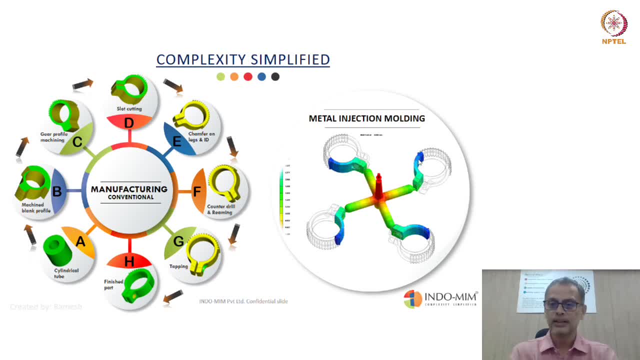 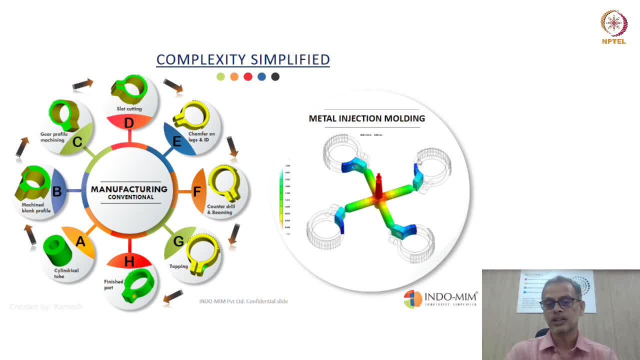 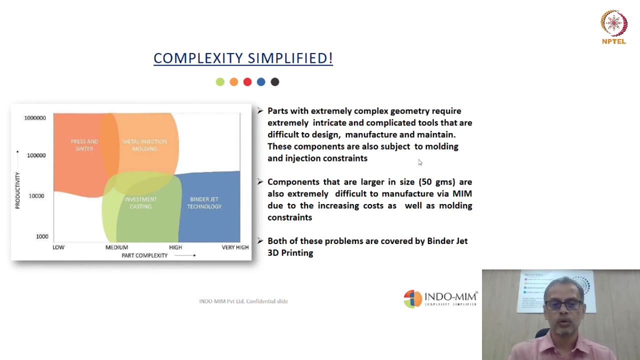 steps eliminated and convert that into a single process called metal injection molding. This specific component is just finished at the metal injection molding without the need of any post-mIMP secondary process. Now, what kind of applications or what kind of windows of opportunities does metal injection molding offer? So here is a slide that gives you productivity on the y-axis. 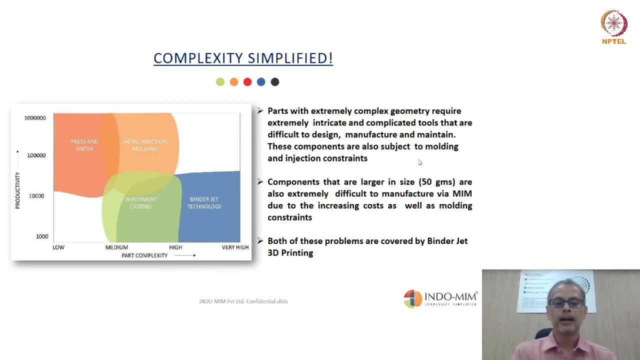 which means the quantity. So here is a slide that gives you productivity on the y-axis, which means the quantity that you need annually, and part complexity on the x-axis, where we are spanning the complexity right from low to medium high and going to very high. So, if you can see, 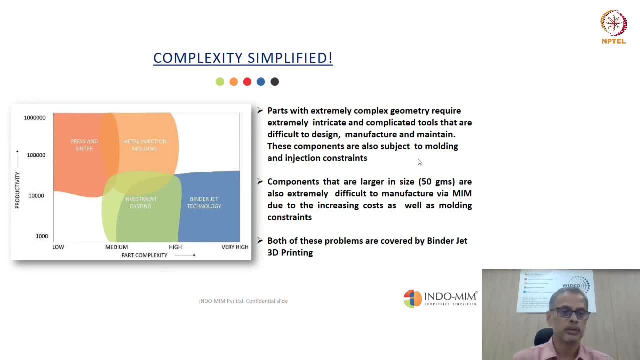 low part complexity and high volume is something which is the domain of press and sinter or powder metallurgy. If the volume is less, that means the quantities are less, whereas the part complexity is medium or high, you would end up using investment casting, And if the medium to high complexity is available for the part as well as the productivity, 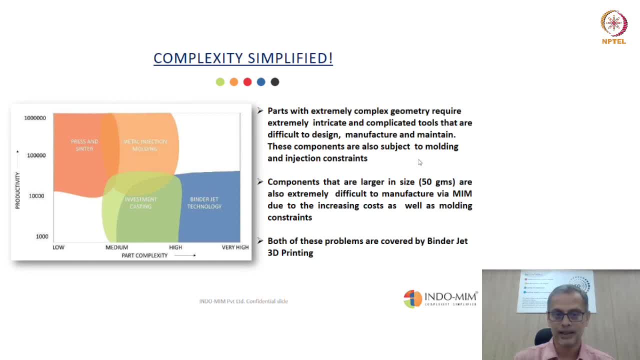 is high or the quantity is high. that is when you end up using metal injection molding. So basically, we are talking about complexity as the prerequisite for metal injection molding to be favorable. Yet another new emerging technology, called binder jet technology, is something which Indomium has really got into, and that is for the area of high or very high complexity, with low 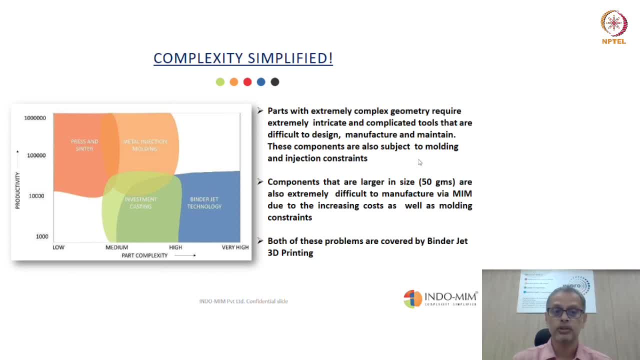 volumes. So this is the area of high or very high complexity with low volumes. So, if you can see, I briefly mentioned that binder jet technology also uses more or less similar process flow like metal injection molding, just that the molding process is replaced by a printing process. 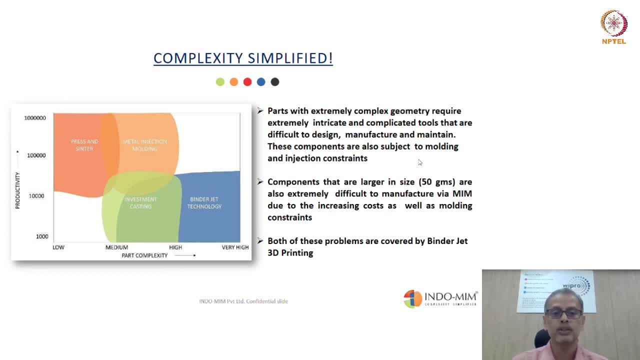 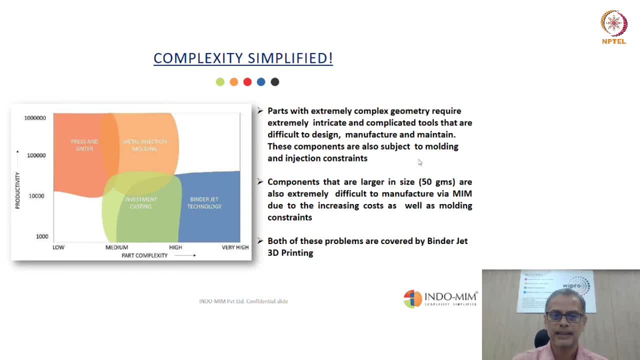 10 grams, 15 grams- that is the weight range of metal injection molded parts. But most of these parts would have at least about 25 to 30 measurable dimensions or critical dimensions on the component drawing. So that is a very, very easier way of identifying part. 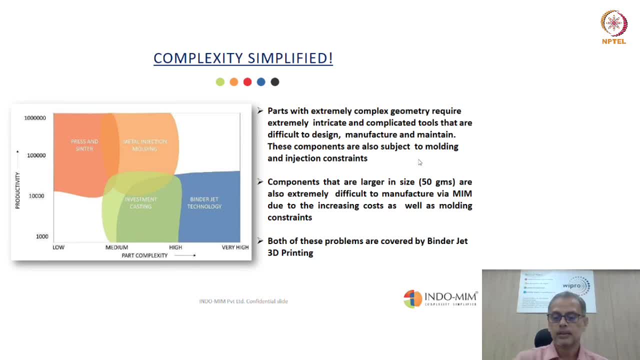 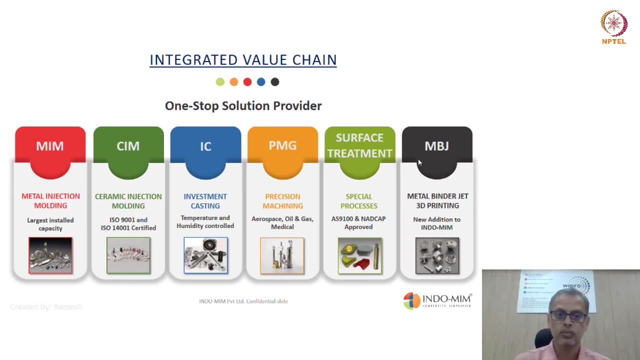 favorable for metal injection molding. So Indomium offers an integrated value chain starting from metal injection molding to ceramic injection molding, investment casting, precision machining, special processes and metal binder jet 3D printing. So we are basically a one-stop solution provider. 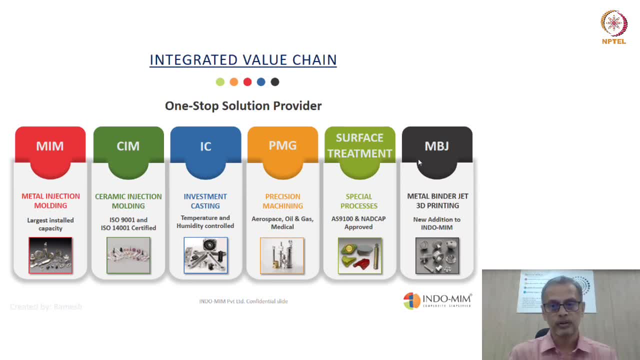 who is able to offer all these solutions for all of our global customers. 92 percent of our sales is exports and Indomium is a very popular and very credible name to reckon with across the globe in the manufacturing space. So Indomium is a very popular and very credible name to reckon with across the globe in the manufacturing space.